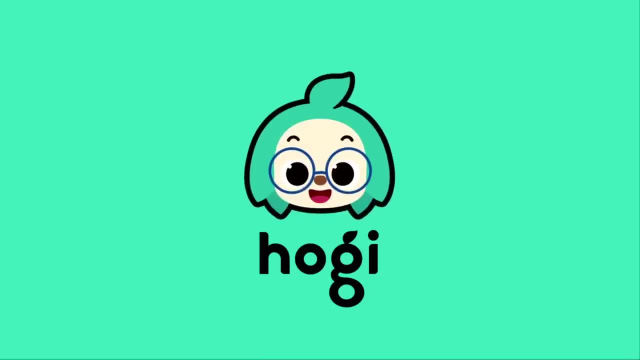 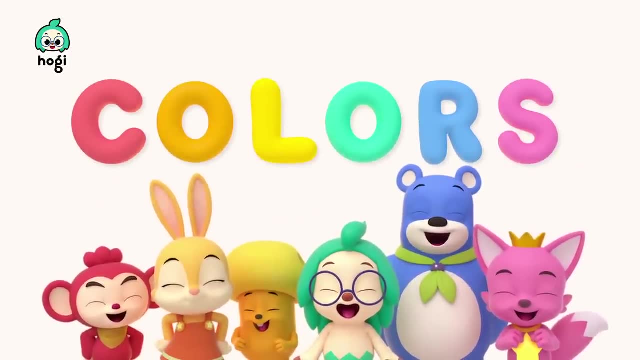 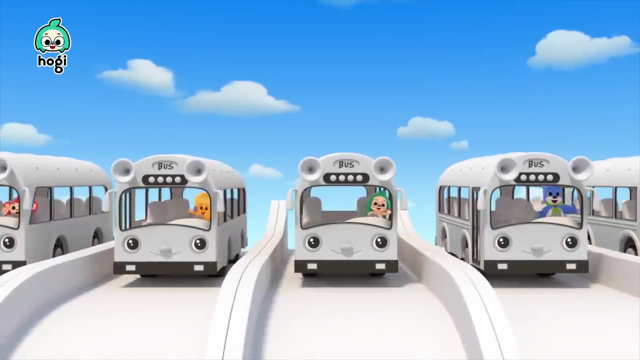 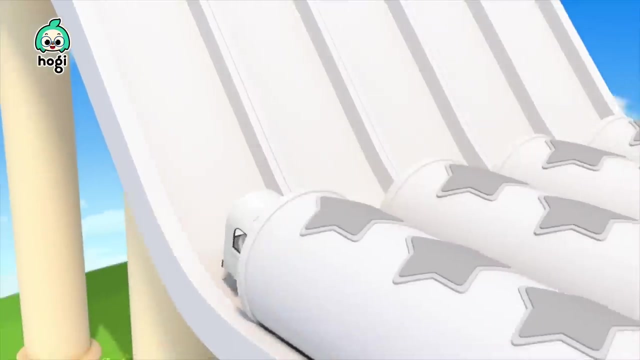 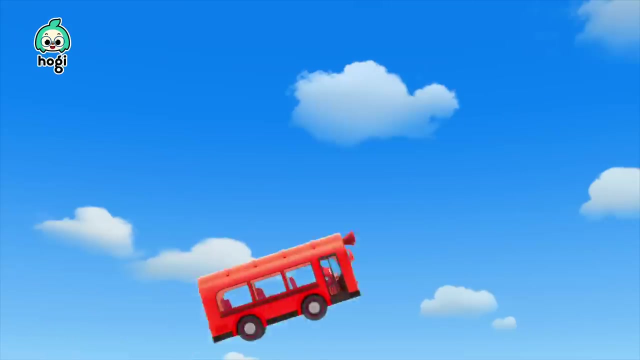 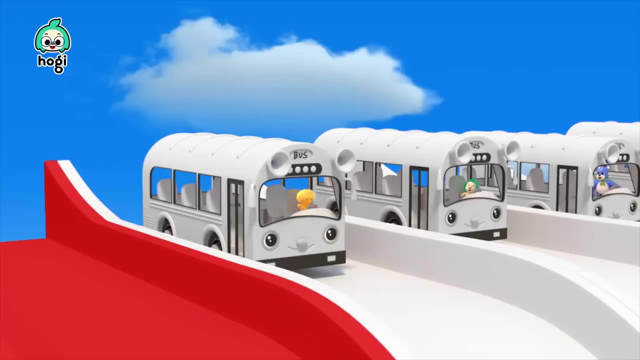 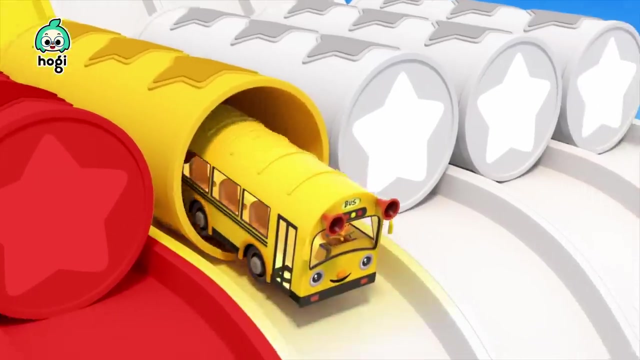 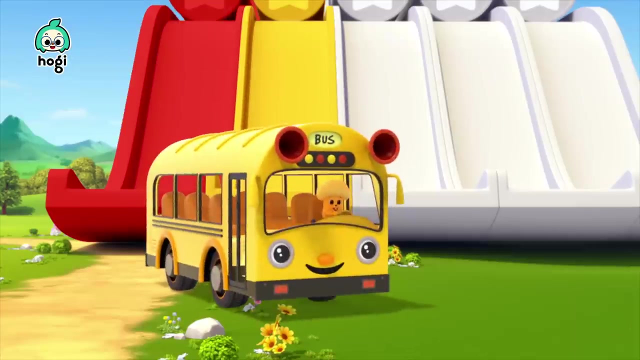 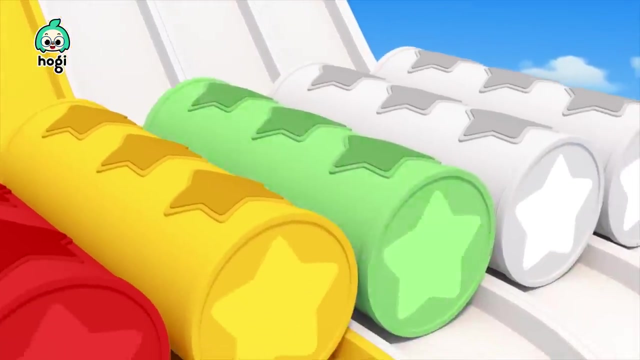 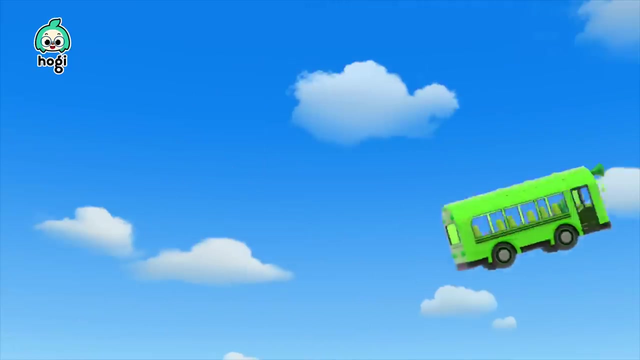 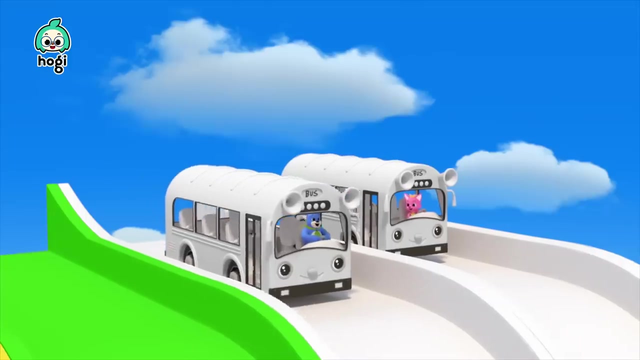 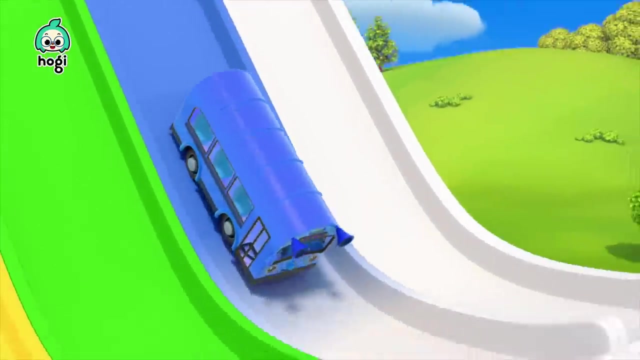 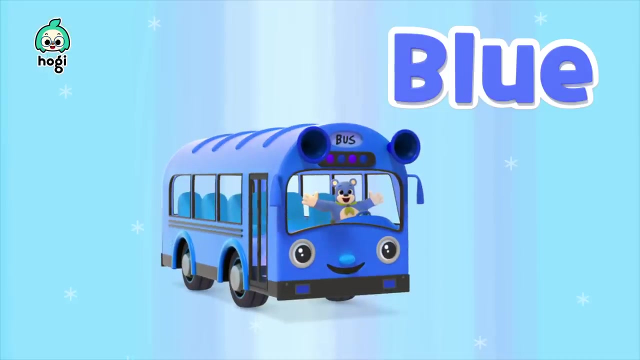 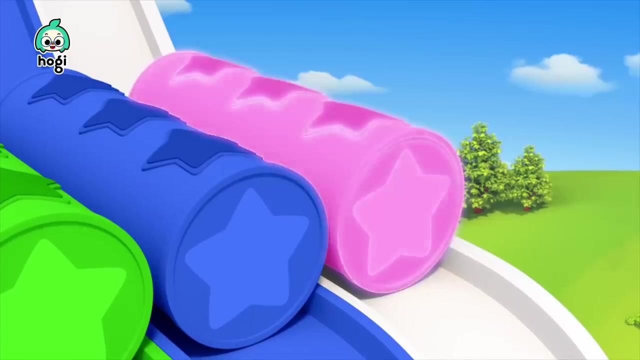 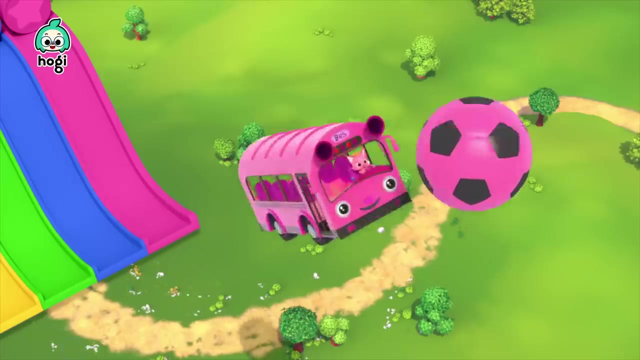 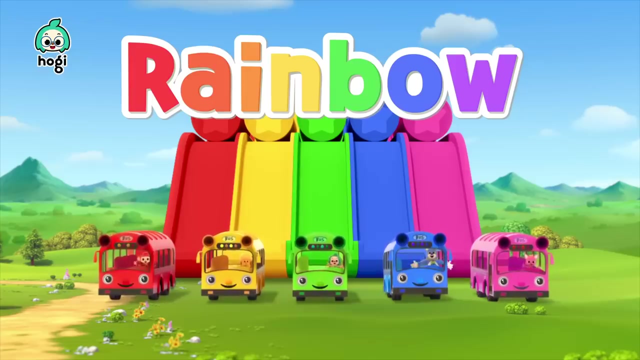 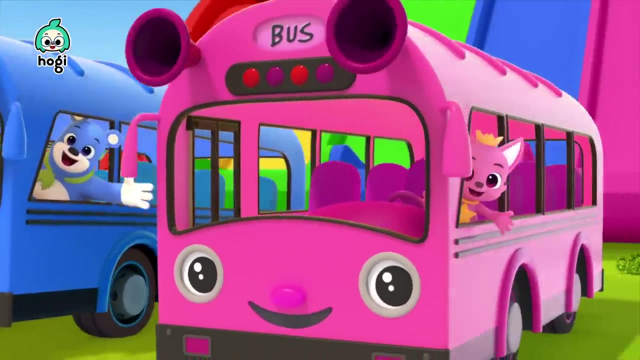 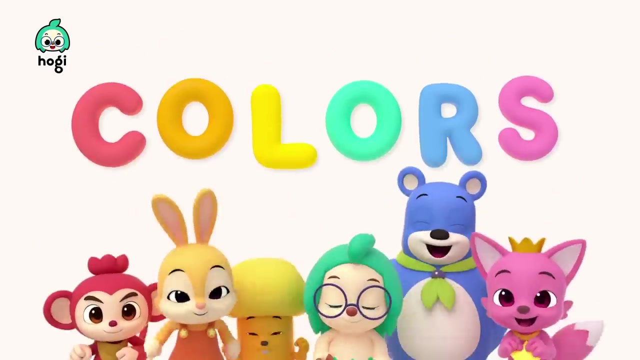 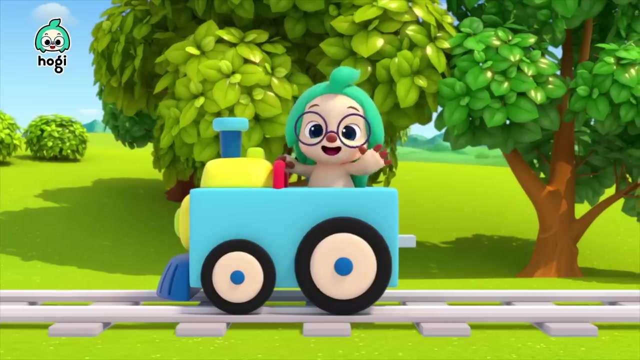 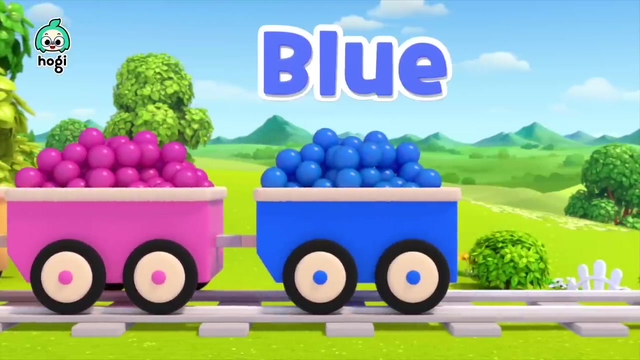 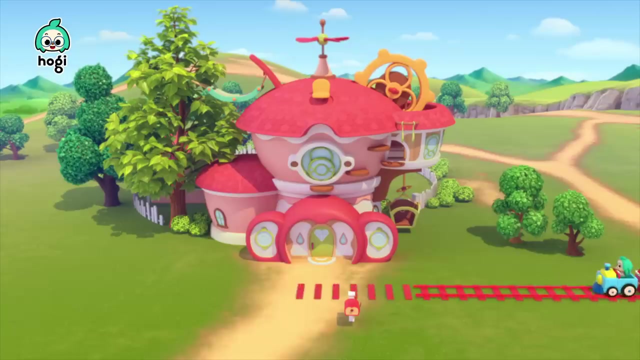 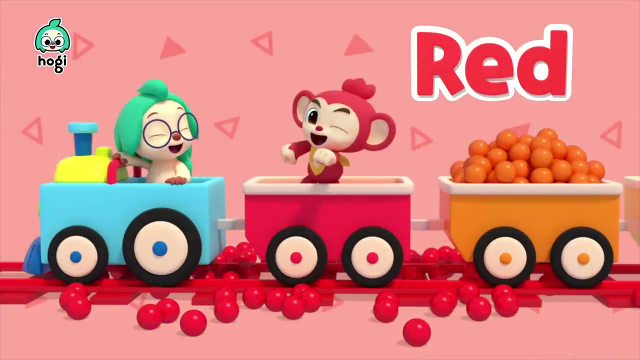 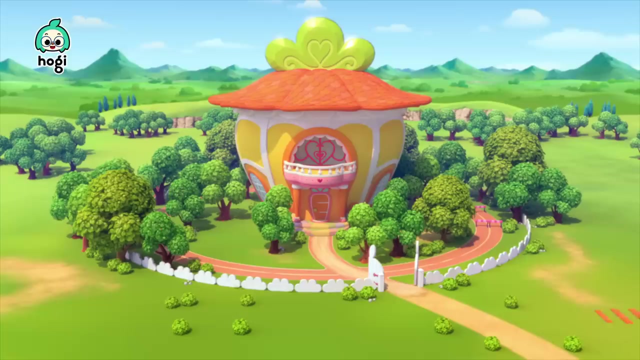 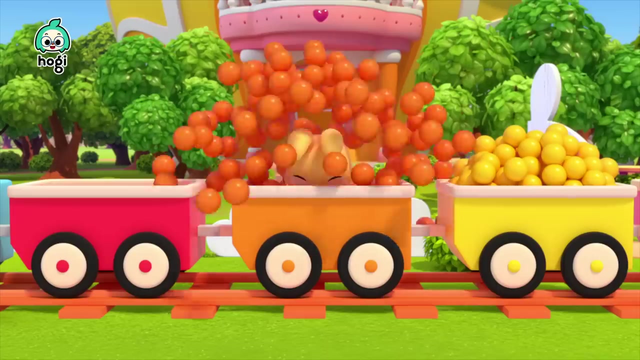 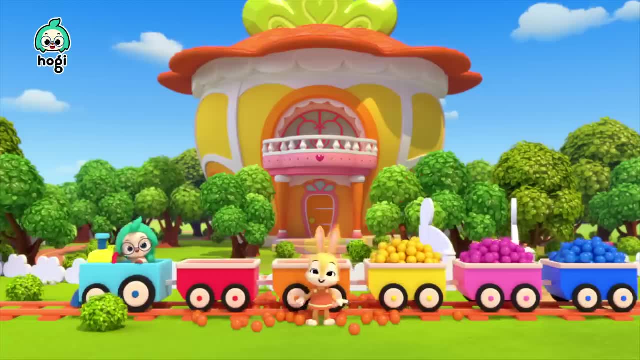 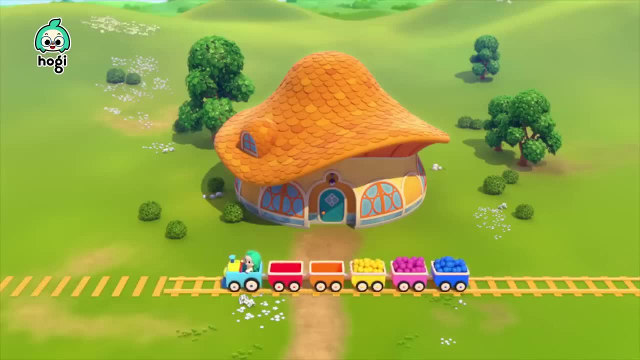 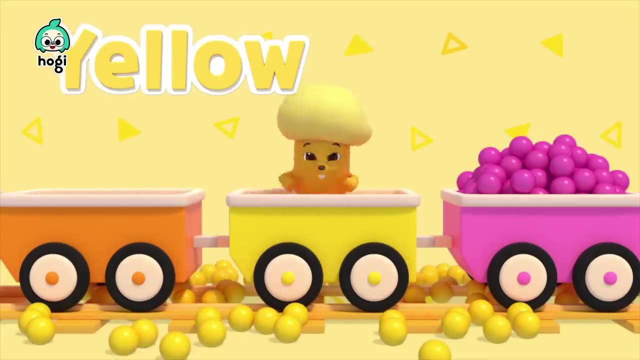 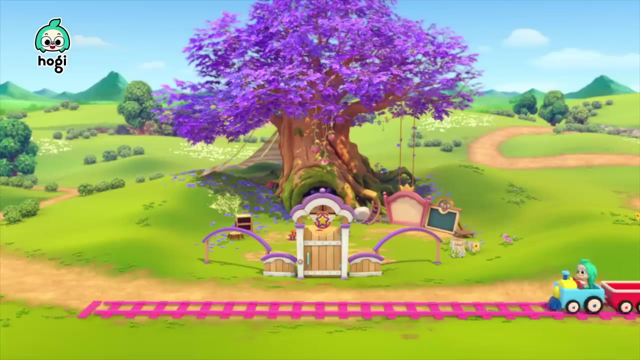 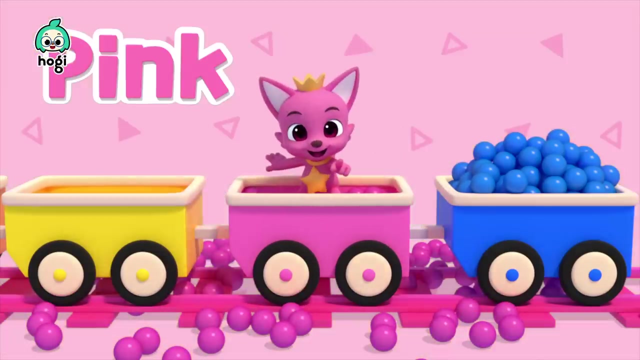 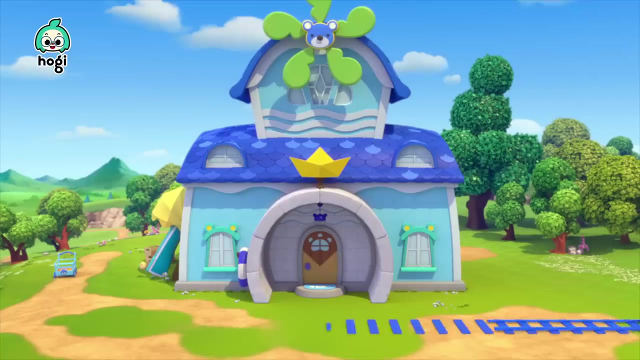 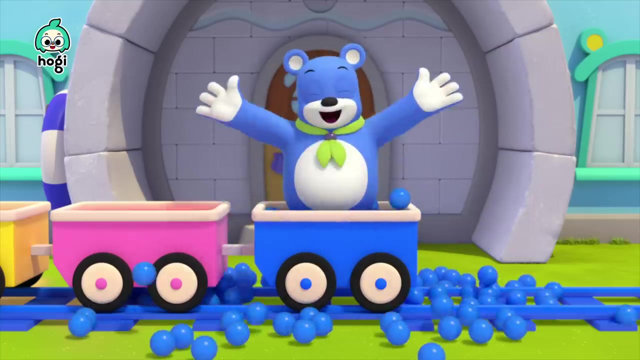 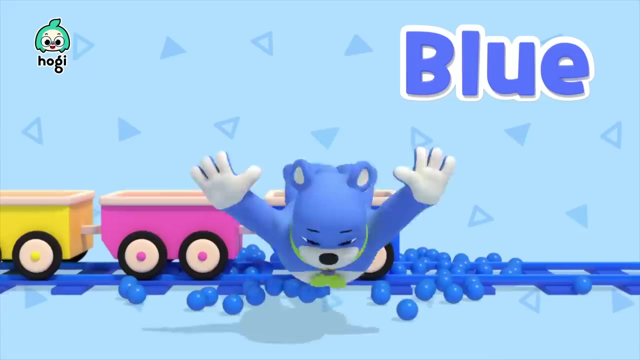 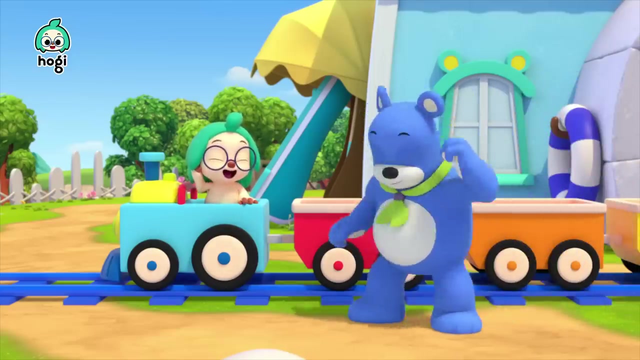 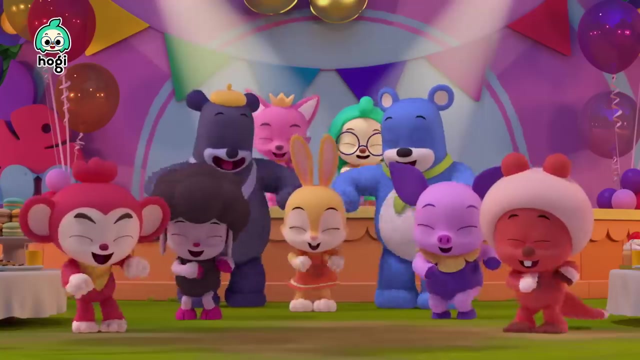 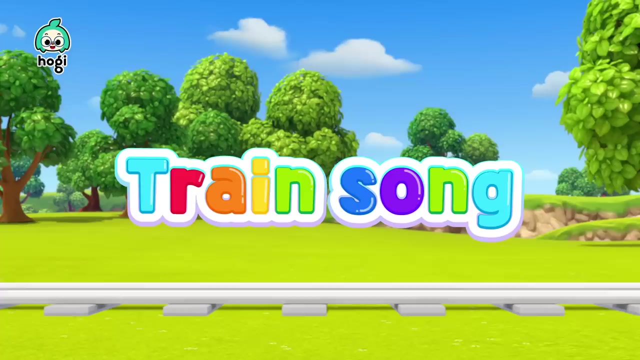 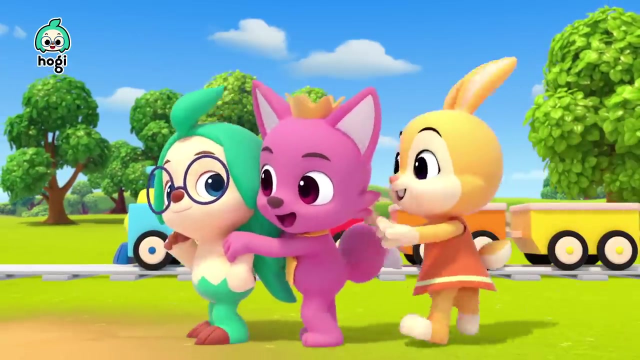 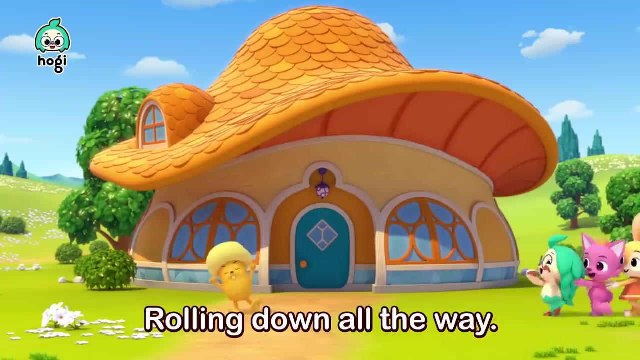 Yellow, Pink, Blue. Yeah, Sing along with Pinkfong and Hoagie All aboard: Chugga chugga choo choo choo, Chugga chugga choo, choo choo, Rolling down all the way, Anytime, anywhere. 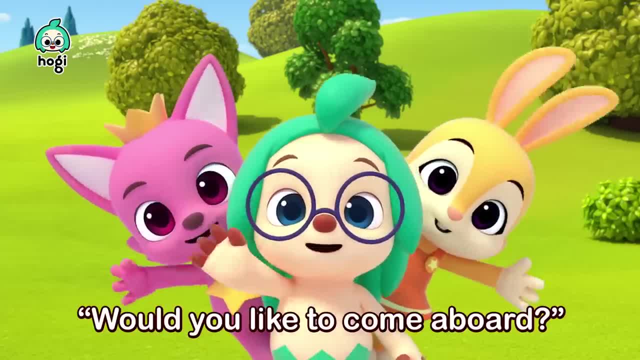 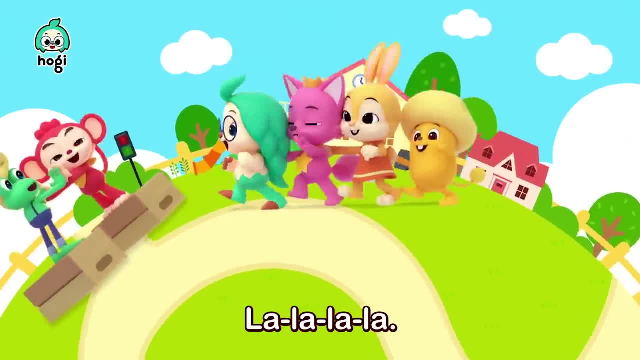 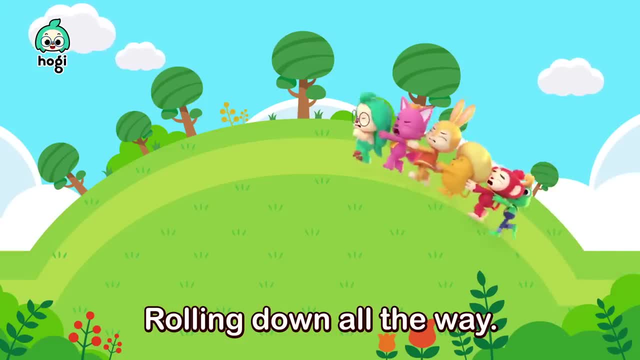 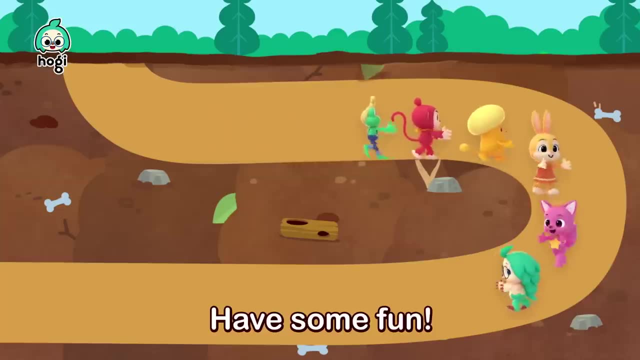 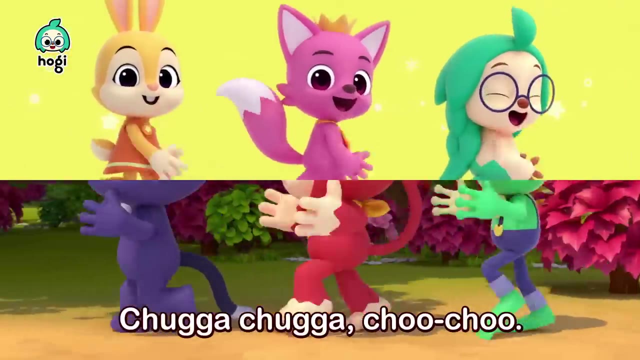 Chugga chugga choo choo tree Rolling down all the way Anytime, anywhere. Let's all ride the train together. Hey, Have some fun, Have some fun. Let's all shout and sing together: Chugga chugga choo choo. 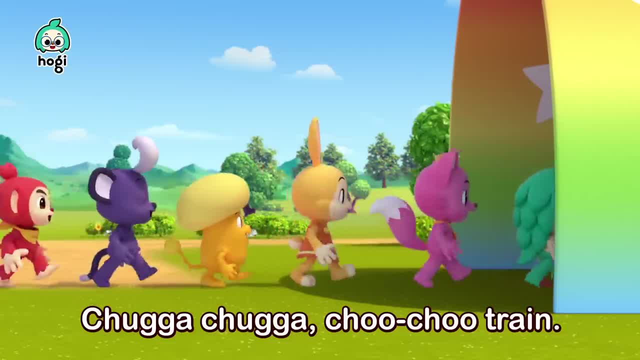 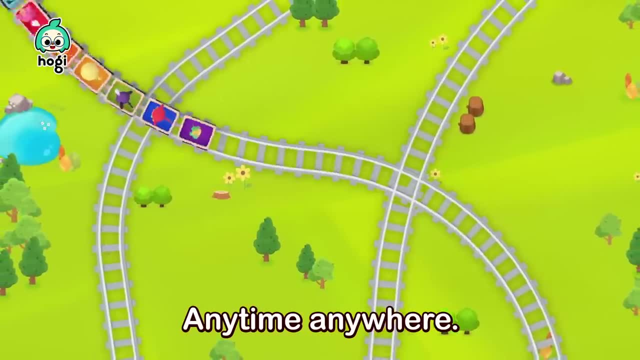 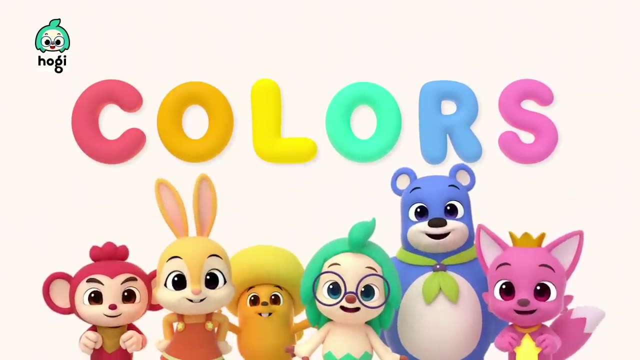 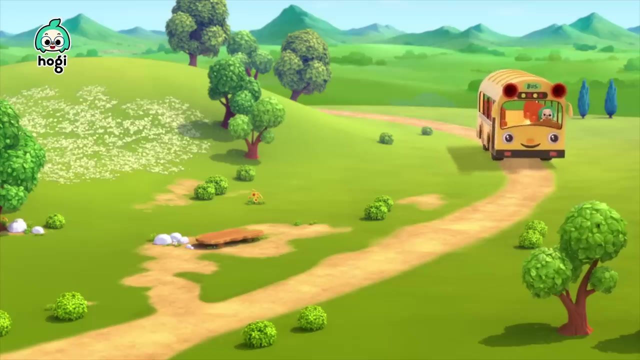 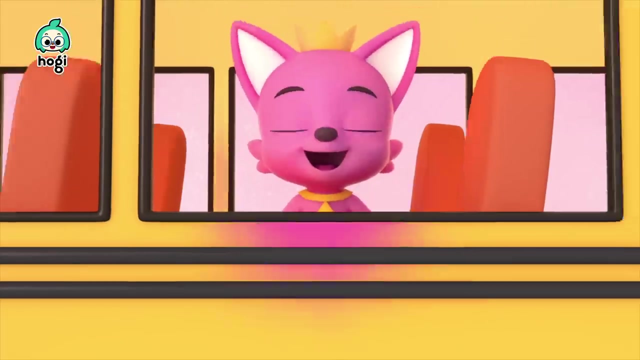 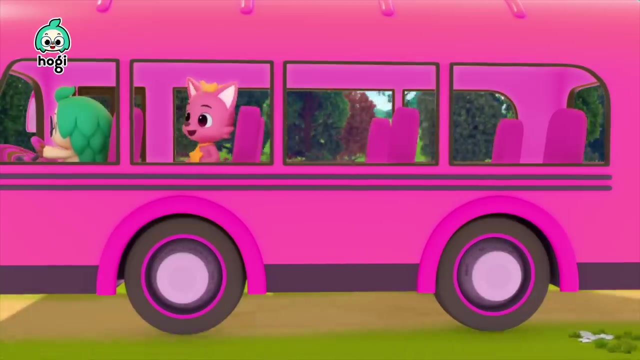 Chugga chugga choo choo choo. Chugga chugga choo choo train. Chugga chugga choo choo train Rolling down all the way, Anytime, anywhere. Yeah, Anything's okay. What a beautiful thing. 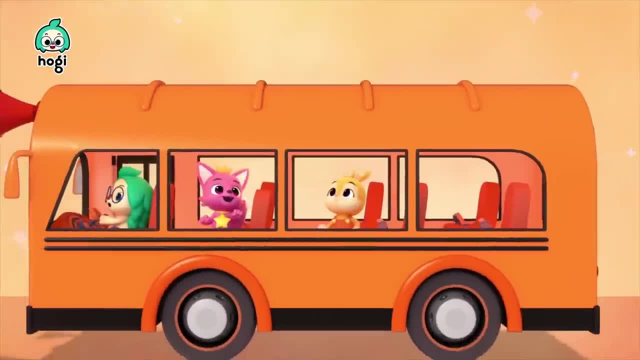 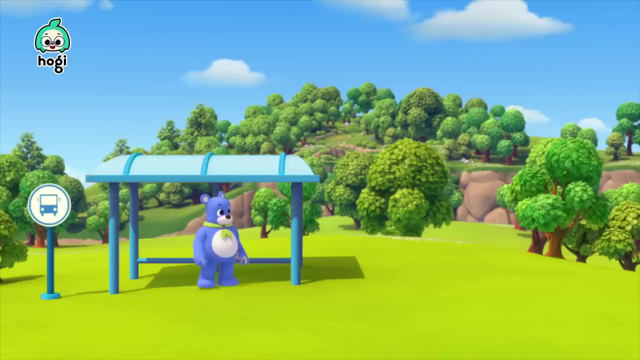 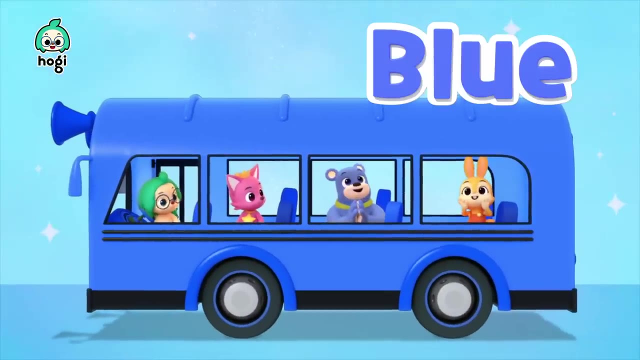 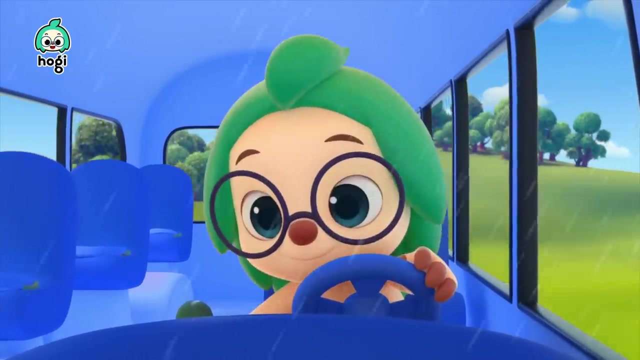 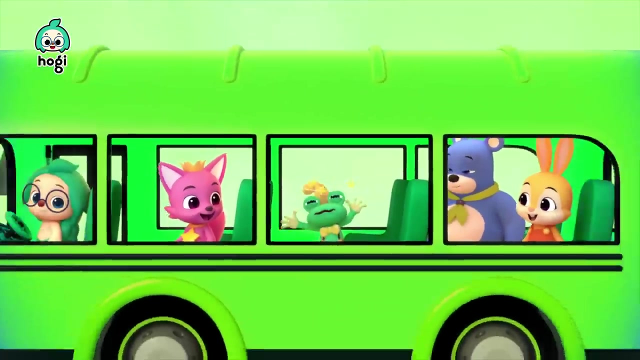 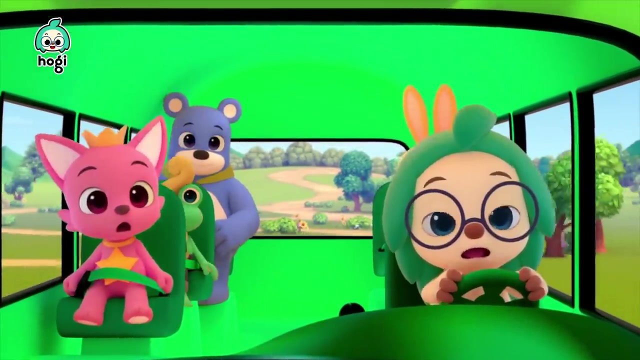 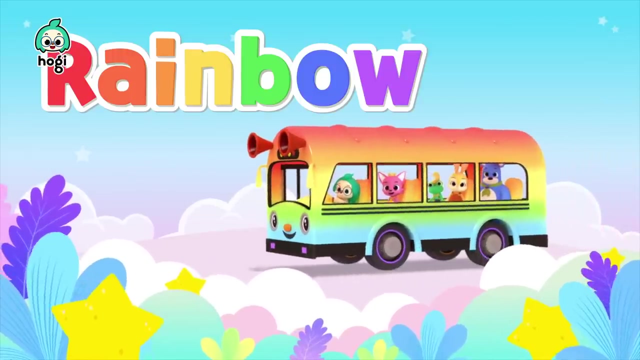 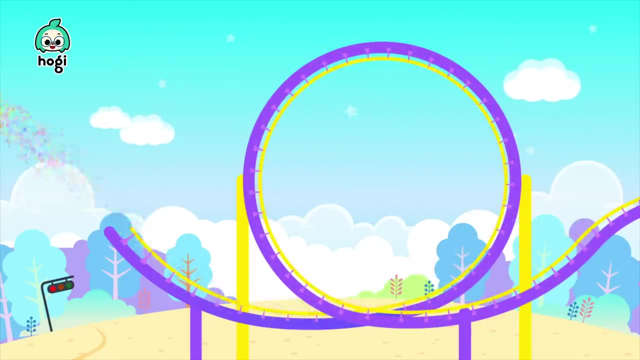 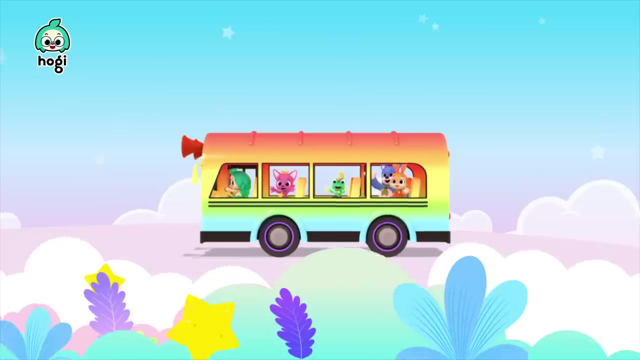 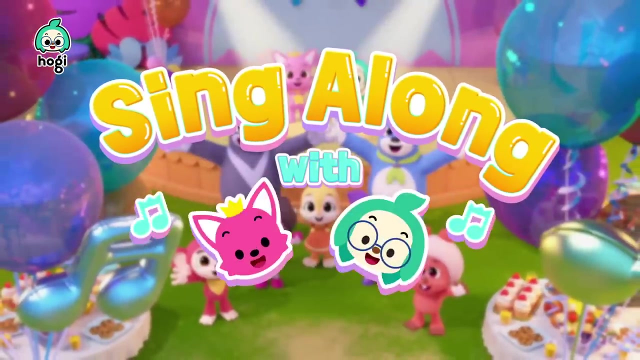 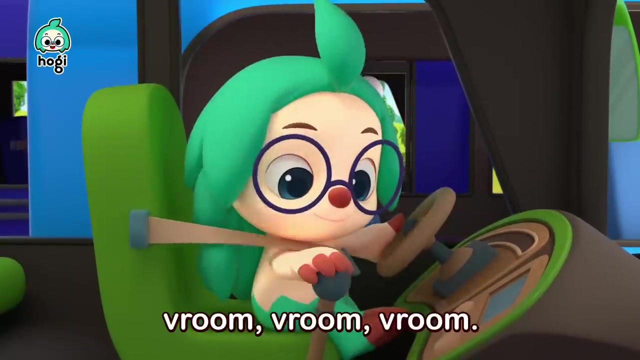 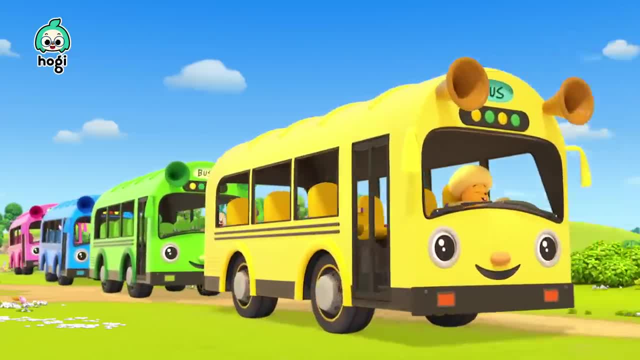 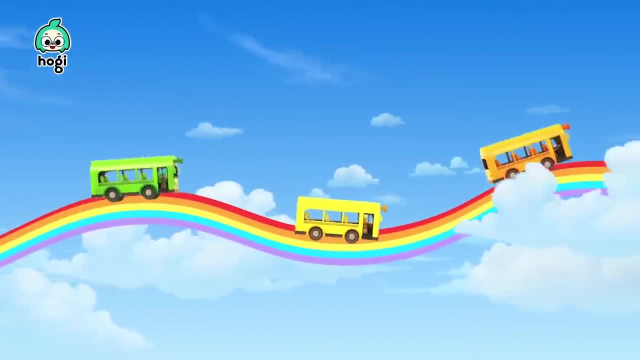 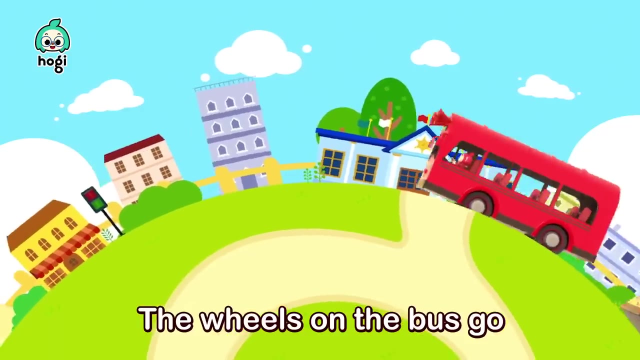 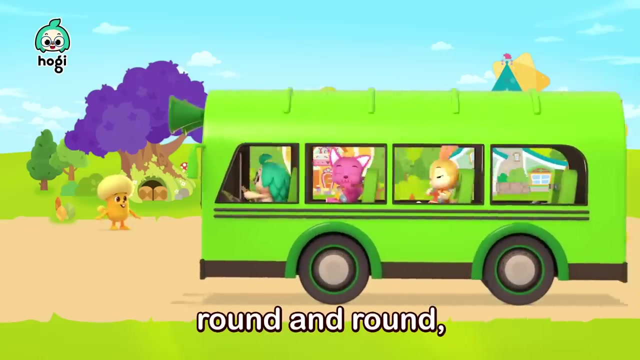 Vroom, Vroom, vroom, vroom. Let's go, Throw wheels on the bus, Go round and round, round and round, round and round. The wheels on the bus go round and round All through the town. The wheels on the bus go round and round, round and round, round and round. 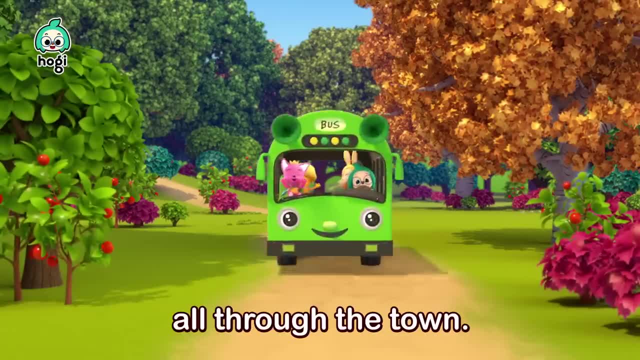 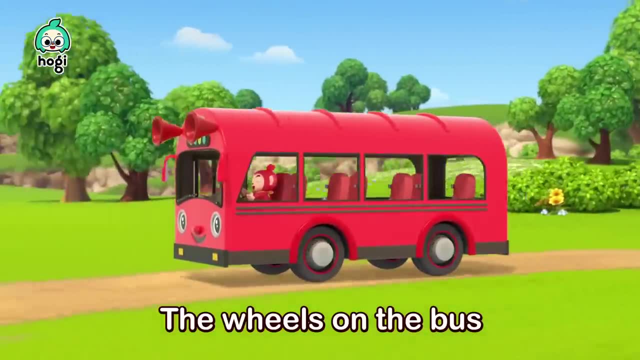 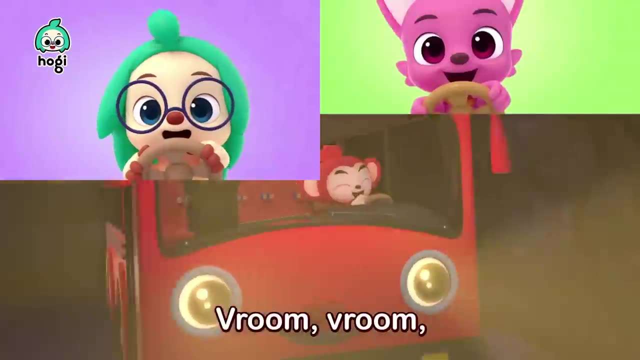 The wheels on the bus go round and round All through the town. The wheels on the bus Round and round. The wheels on the bus, Switch, switch, switch The wheels on the bus, Beep, beep, Vroom, vroom, vroom, vroom, vroom. 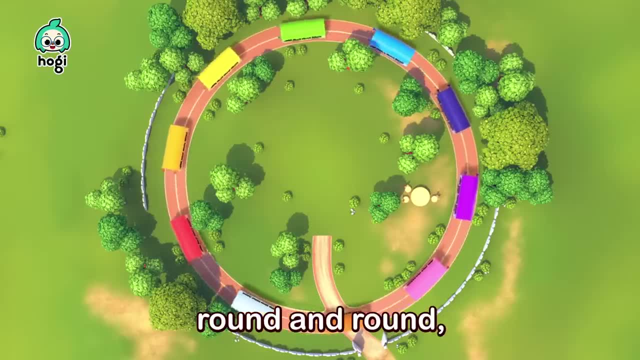 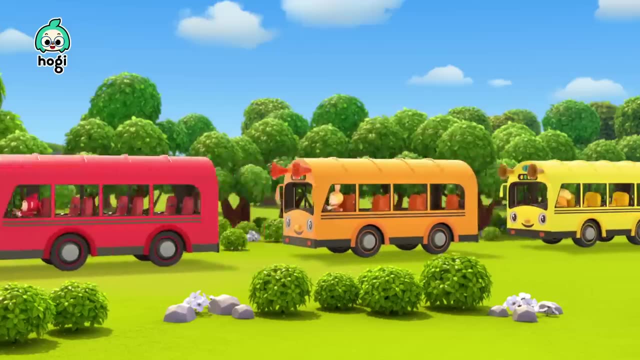 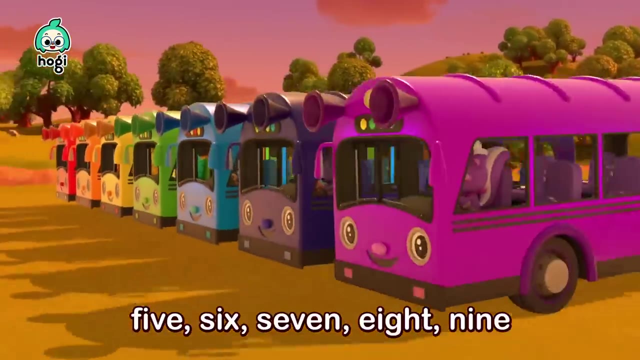 The wheels on the bus go round and round, Round and round, round and round. The wheels on the bus go round and round All through the town. One, two, three, four, five, six, seven, eight, nine And ten Go round and round and round. 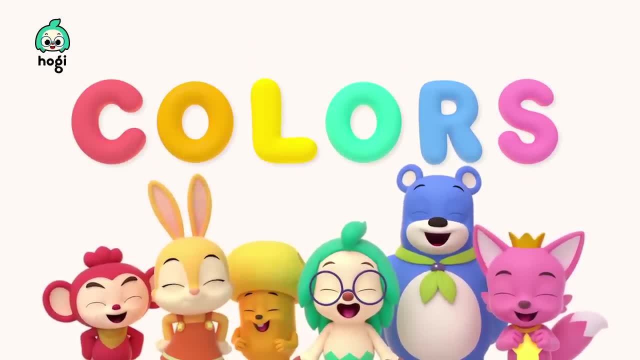 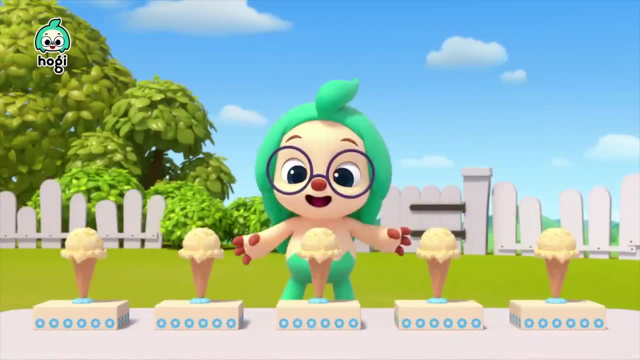 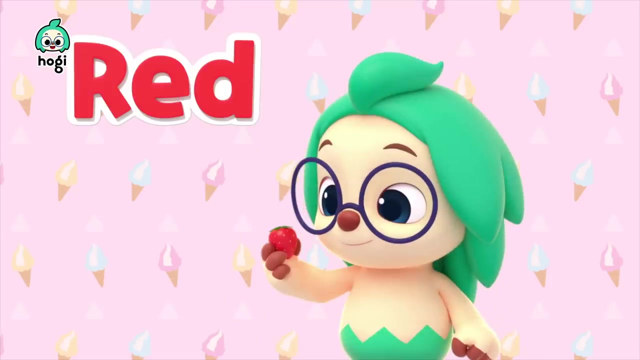 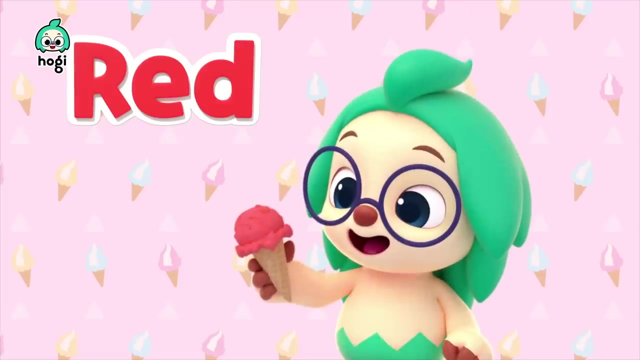 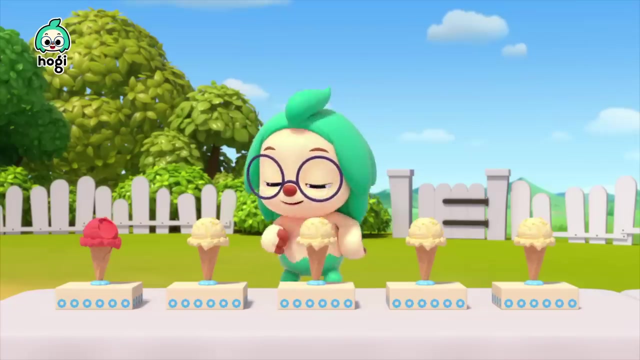 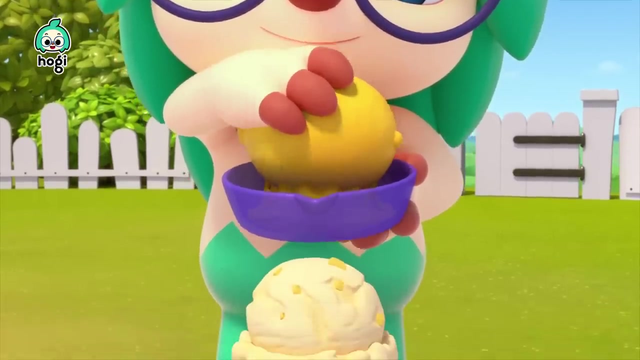 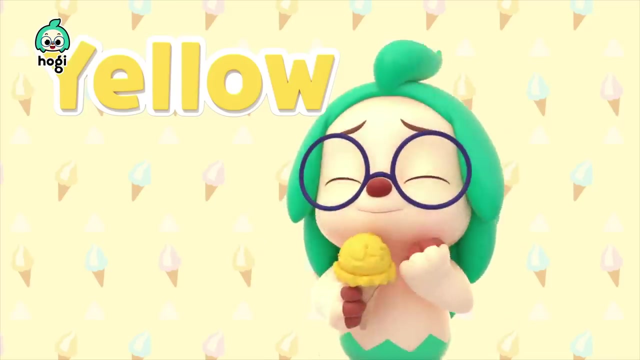 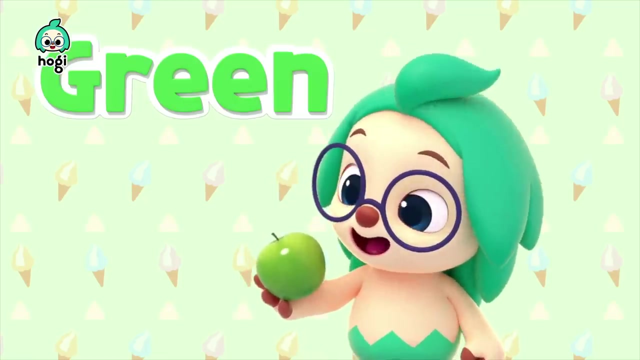 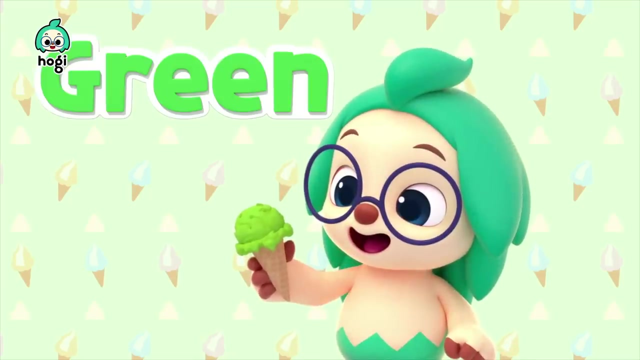 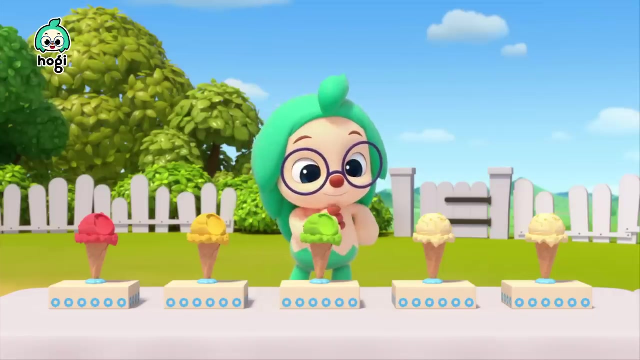 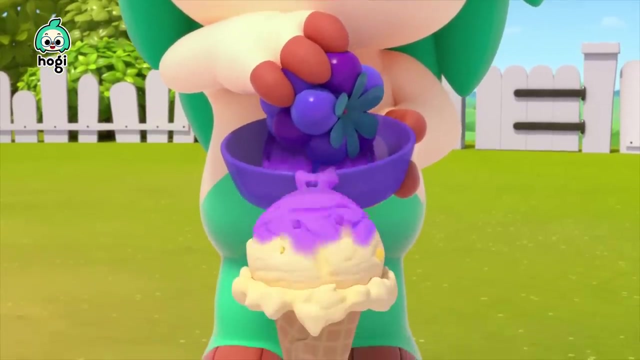 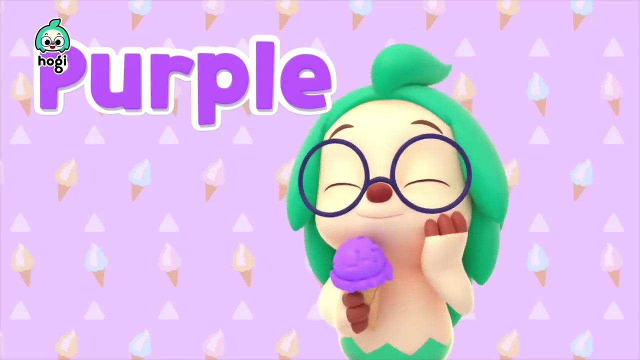 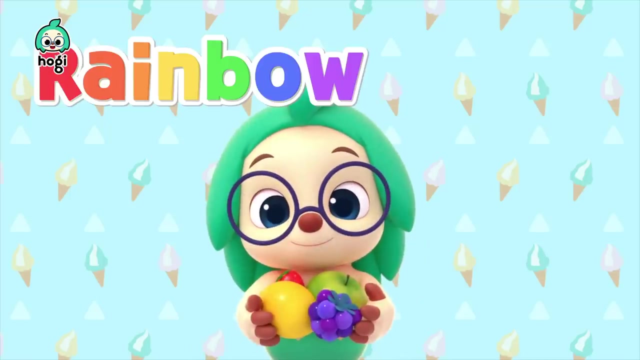 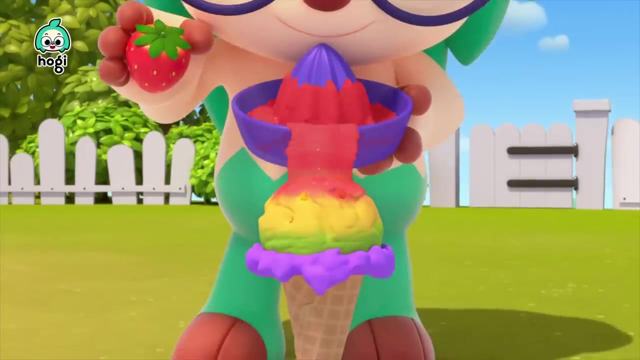 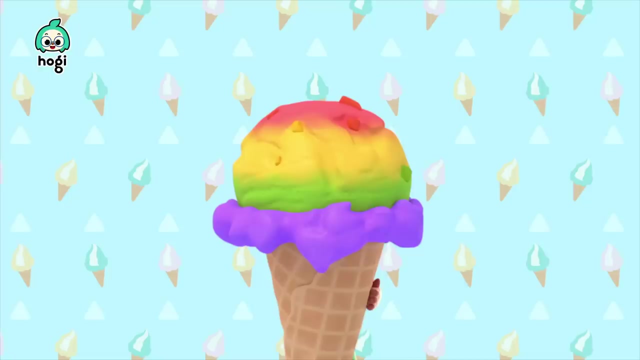 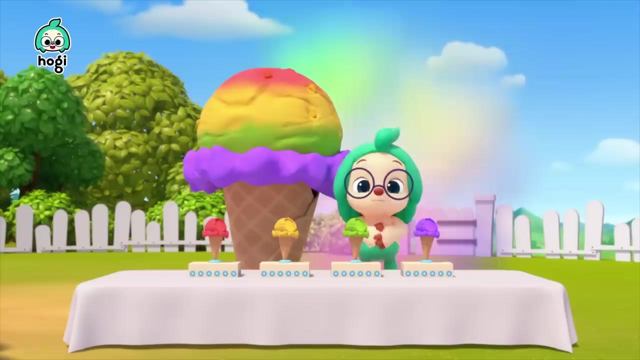 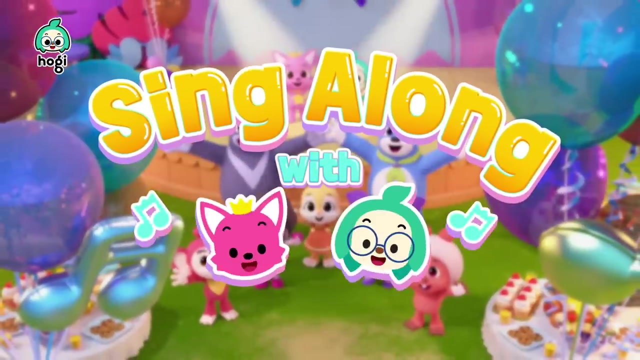 Colors, colors, colors colors: Red, Red, Yellow, Green, Green, Oh, Purple, Purple, Rainbow, Yellow, Blue, Wow, Rainbow, Hahaha, Hahaha, Uh, Oh, Hahaha. Sing along with Pinkfong and Hoagie. Fong and Hoagie. 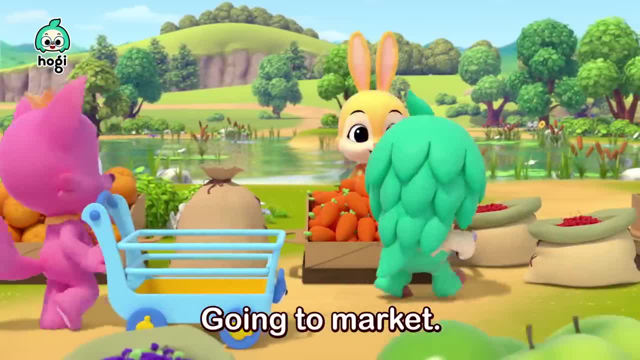 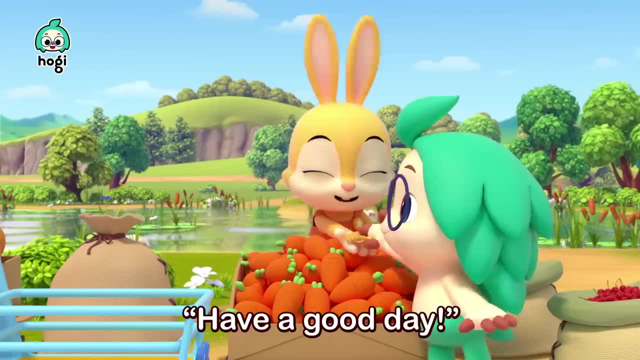 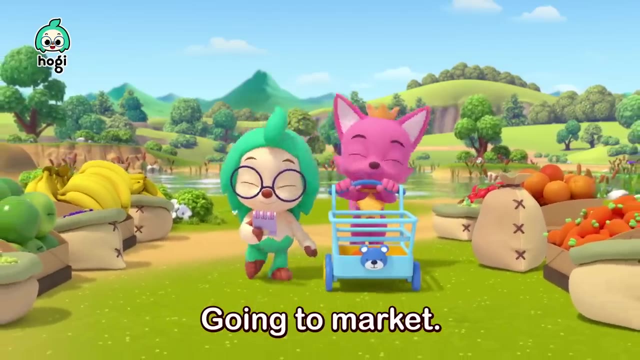 Going to market. going to market: Crunchy crunchy carrots. Put them in our shopping cart. We're taking them home. Have a good day, Thank you. Thank you Bye. Going to market. going to market: Well done, Crunchy crunchy carrots. 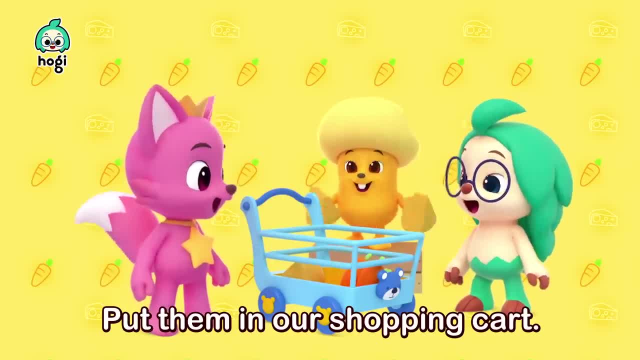 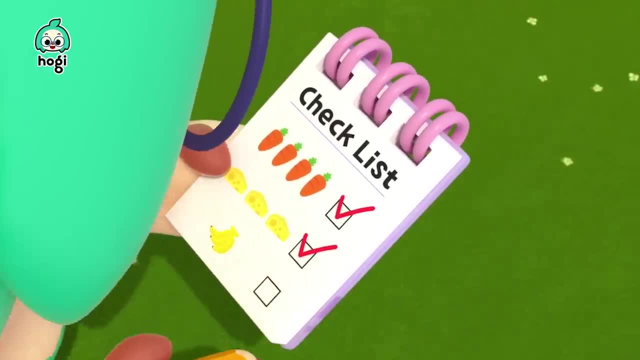 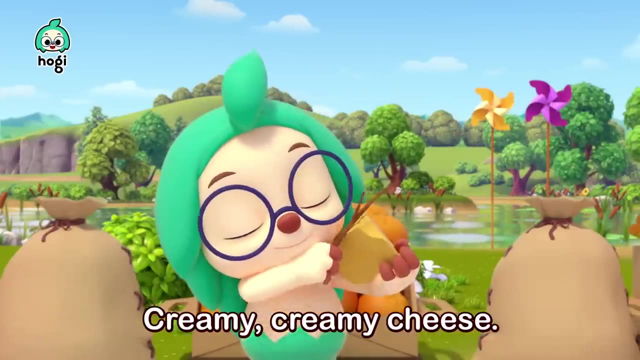 Creamy creamy cheese. Put them in our shopping cart, We're taking them home. Yay, Bye, Bye. Going to market. going to market. Crunchy, crunchy carrots. Creamy creamy cheese, Long, long bananas. Put them in our shopping cart, We're taking them home. 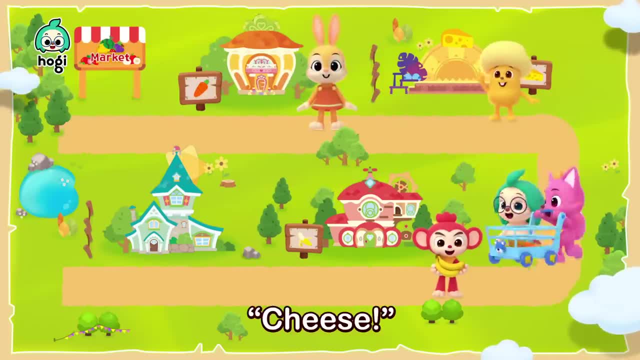 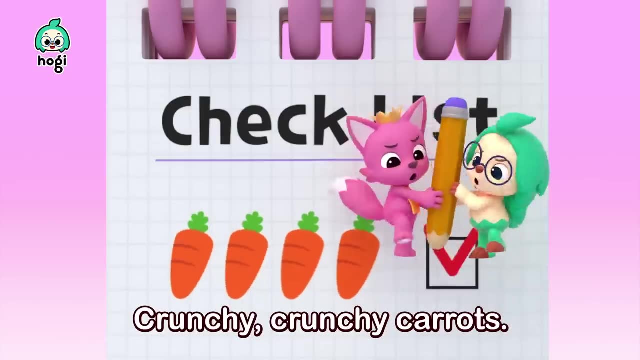 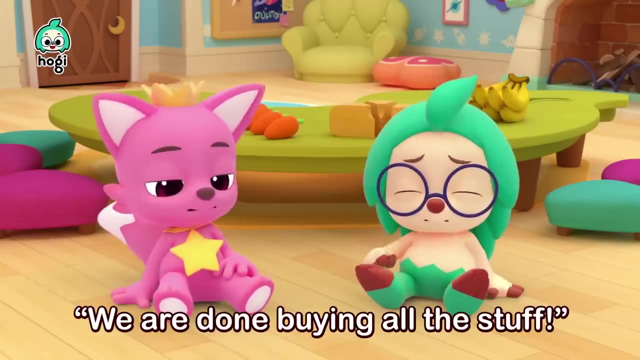 Carrots, Cheese And bananas Going back home, Going back home, Crunchy, crunchy carrots, Creamy creamy cheese, Long, long bananas. We are done buying all the stuff. Yay, This is all we need for dinner. Yummy, yummy, yum. 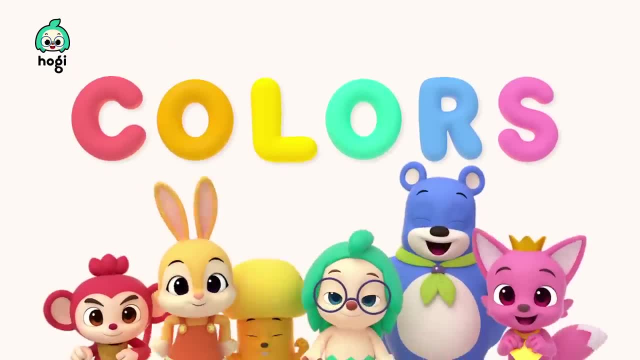 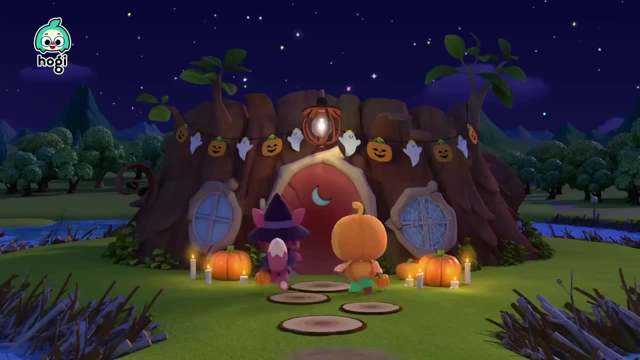 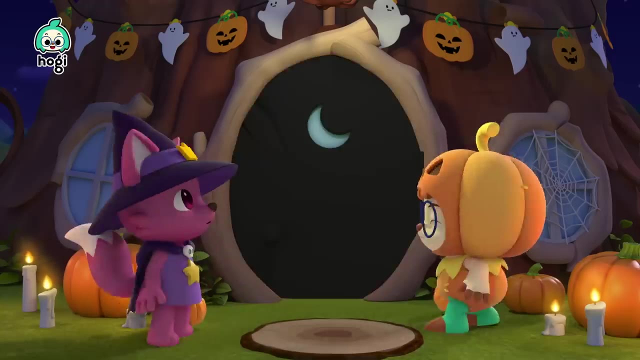 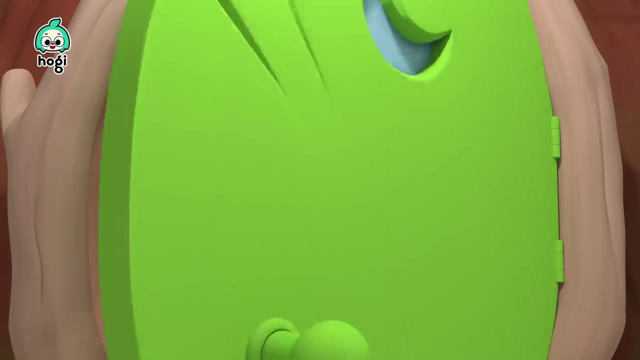 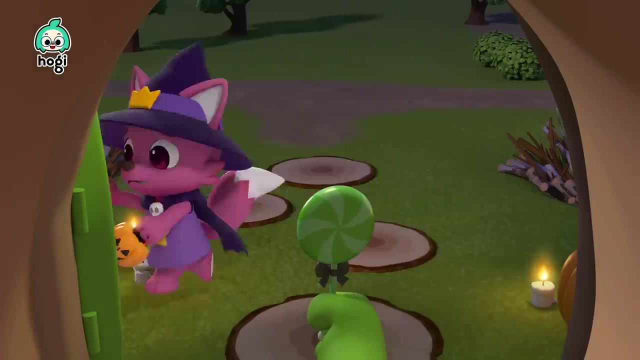 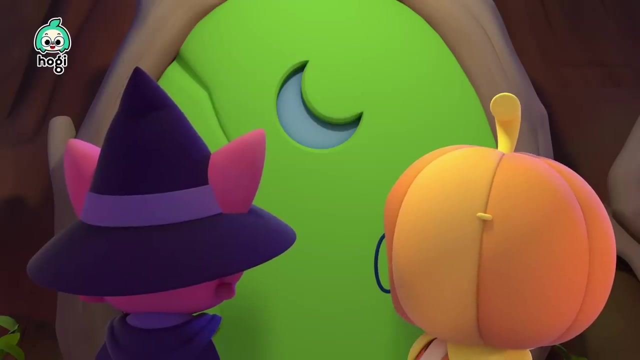 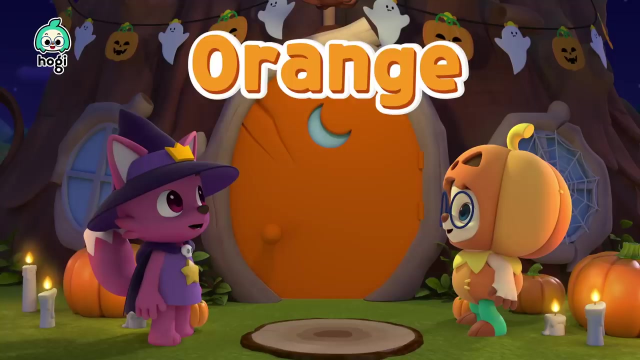 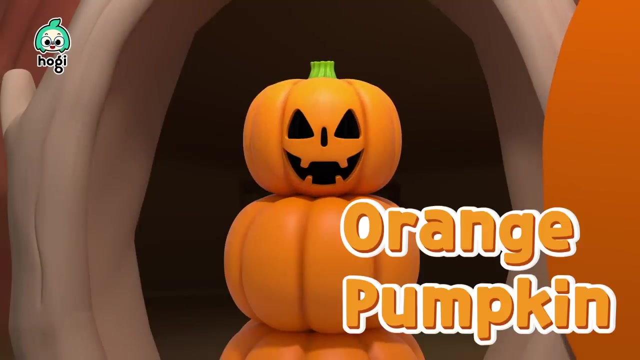 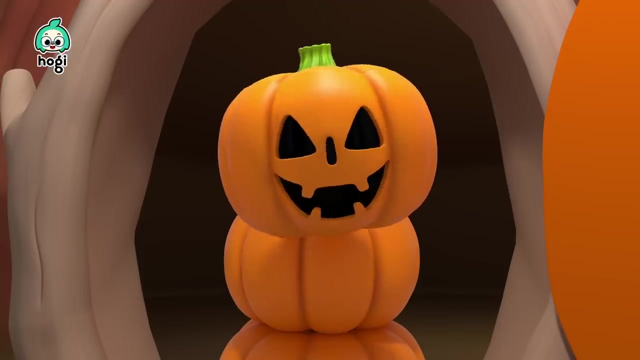 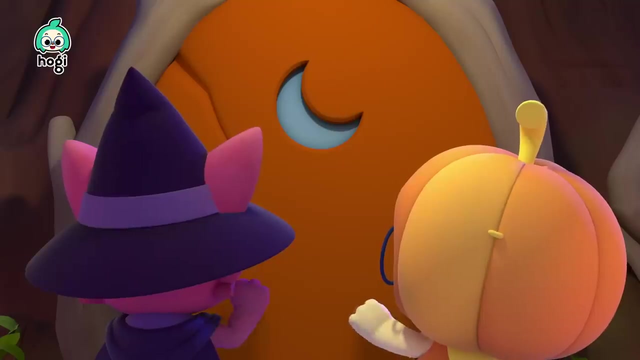 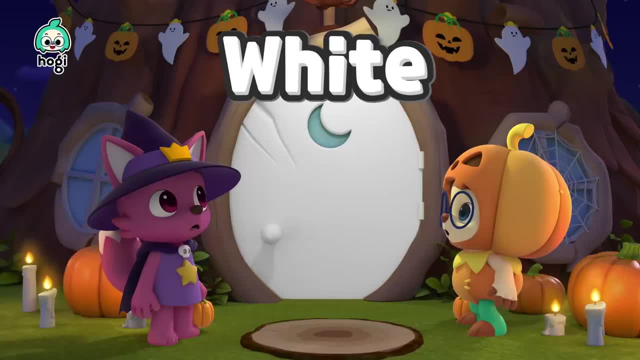 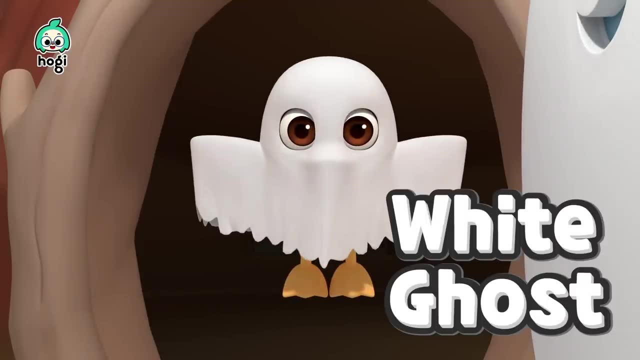 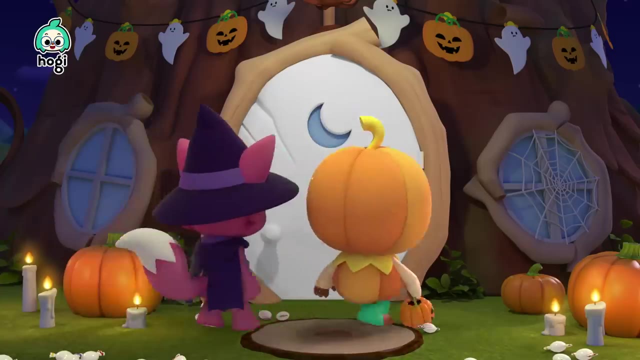 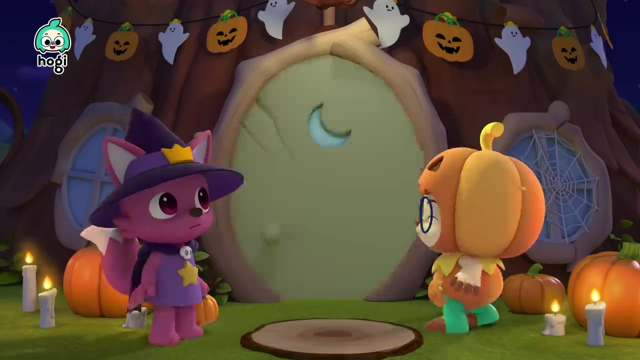 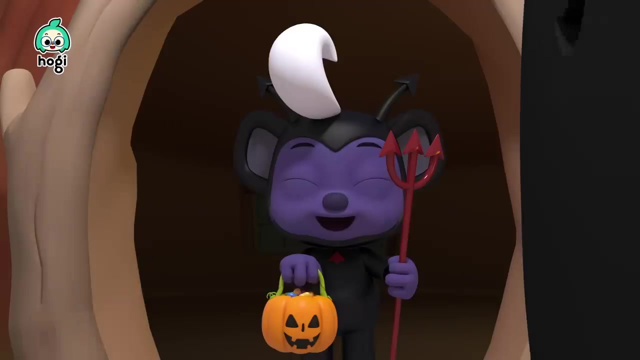 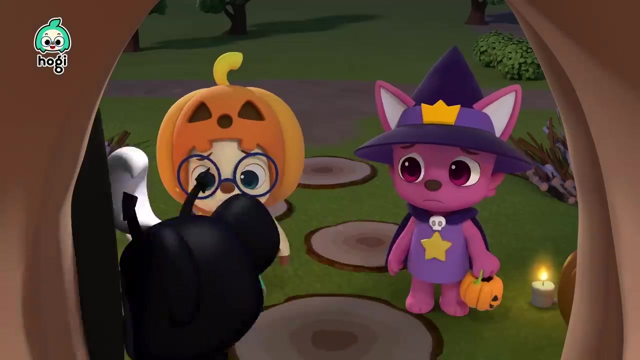 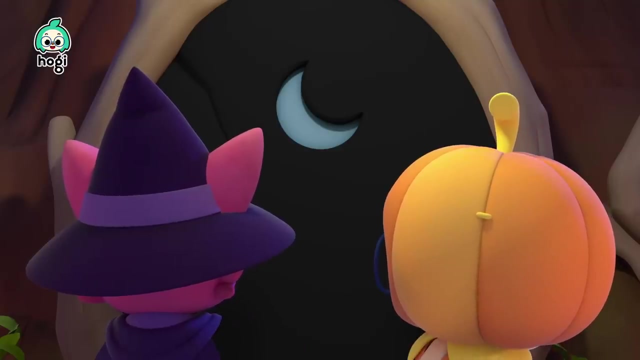 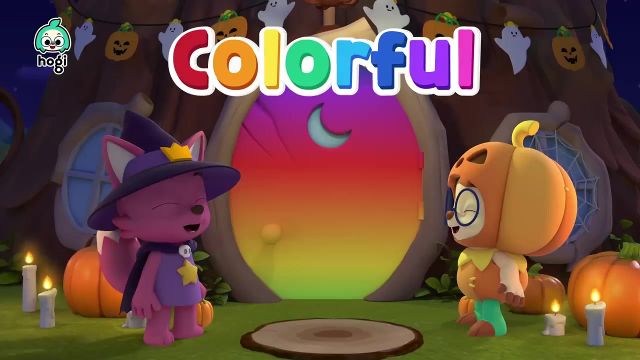 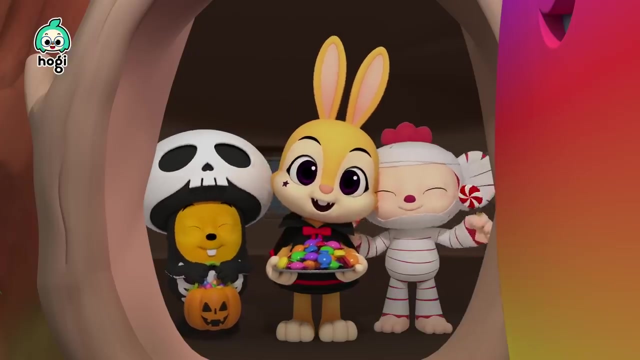 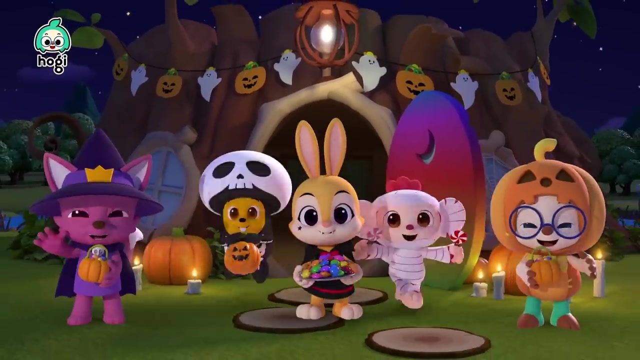 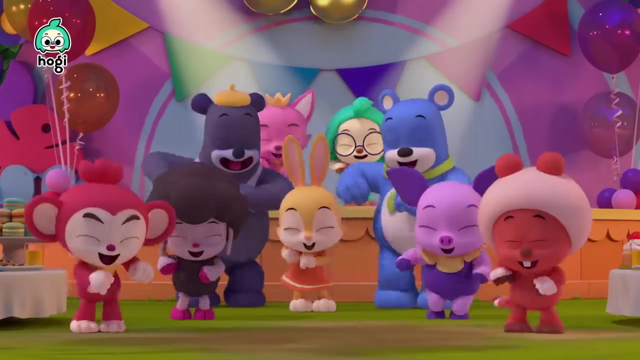 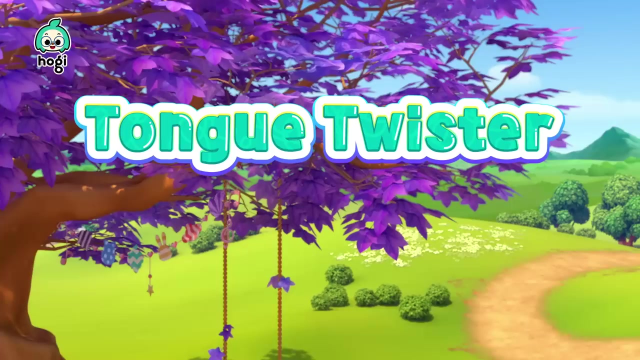 White White ghost Trick-or-treat. Black Black devil Billy Trick-or-treat. Colorful, Colorful candy Candy. Happy Halloween. Happy Halloween. Sing along with Pinkfong and Hoagy. Are you guys ready? 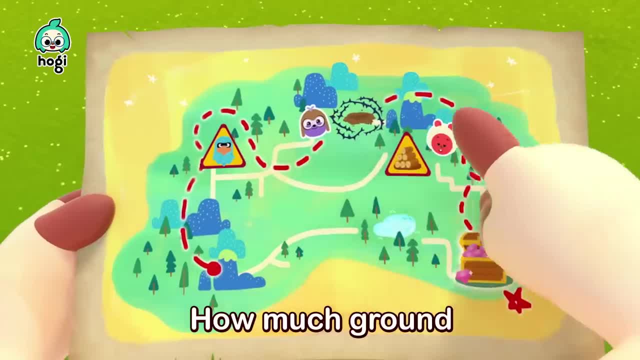 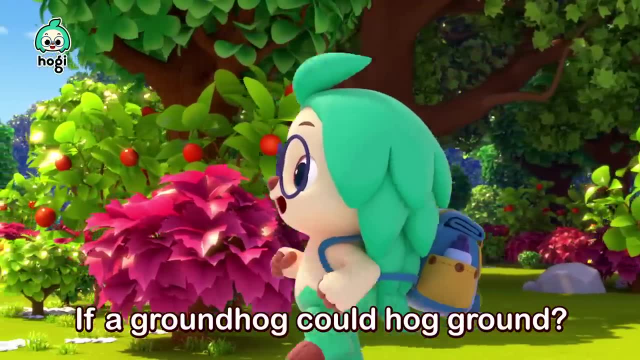 Repeat after me: How much ground would a groundhog need? How much ground would a groundhog need? How much ground would a groundhog need? How much ground would a groundhog hog? If a groundhog could hog ground? If a groundhog could hog ground. 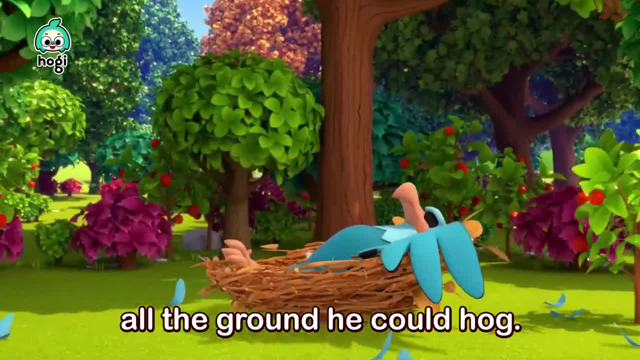 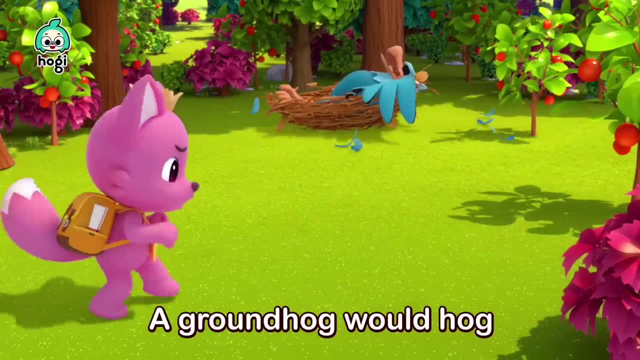 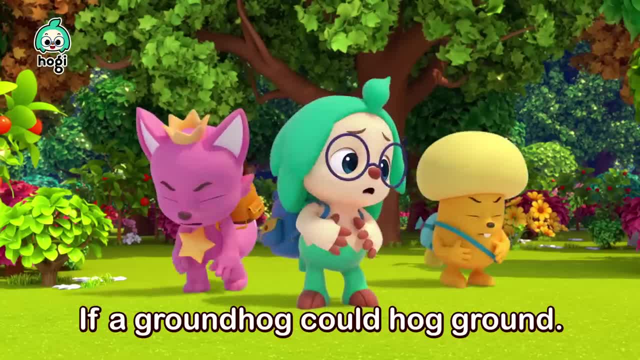 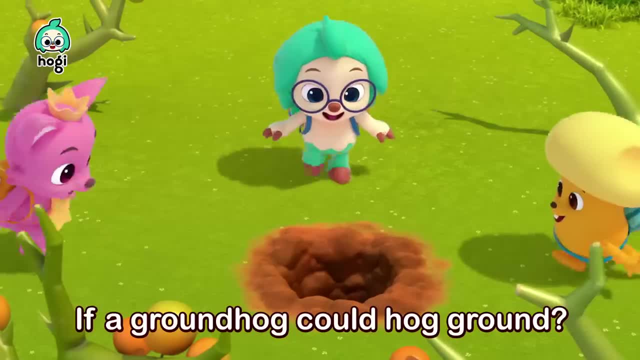 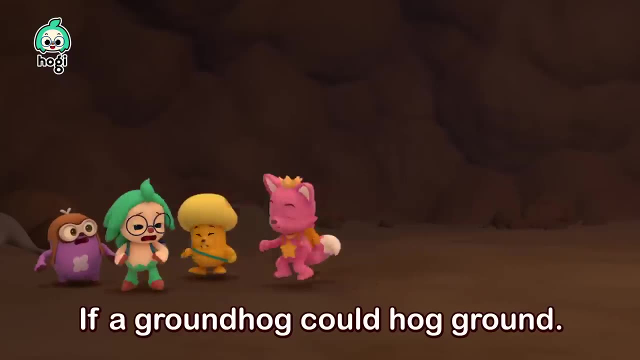 If a groundhog could hog ground, Good, Let's go all the way through. Let's go. How much ground would a groundhog hog If a groundhog could hog ground? A groundhog would hog all the ground he could hog If a groundhog could hog ground. 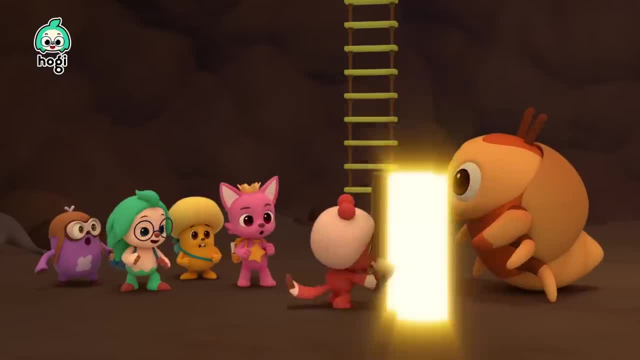 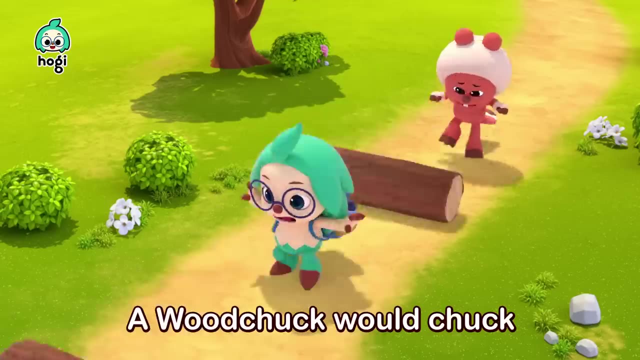 Here comes the real woodchuck. How much wood would a woodchuck chuck? If a woodchuck could chuck wood, A woodchuck would chuck as much as she could. If a woodchuck could chuck wood, A woodchuck would chuck as much as she could. 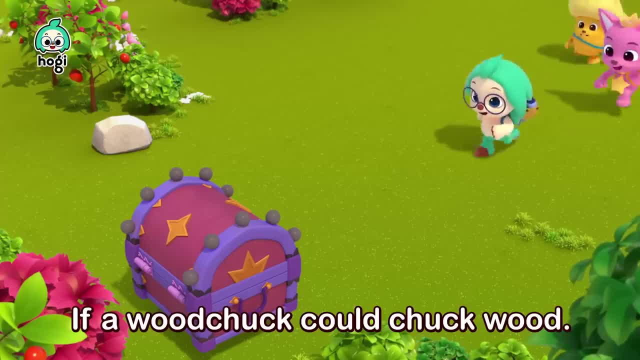 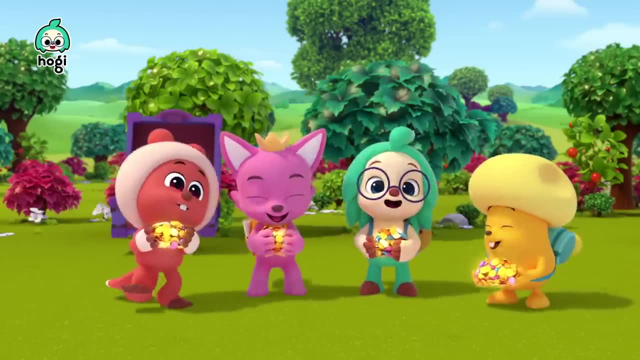 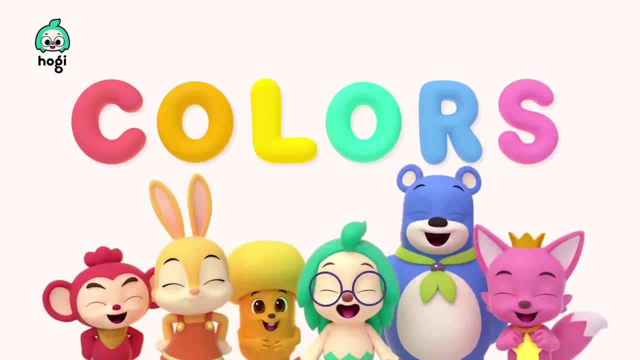 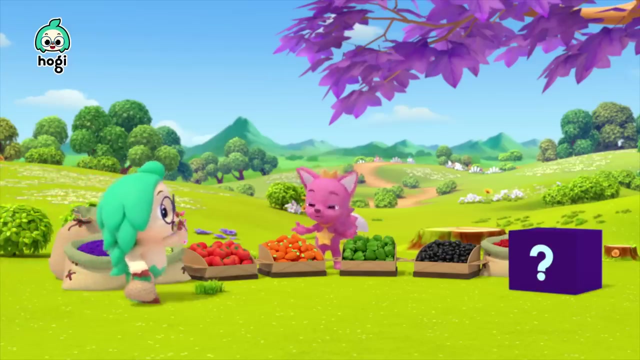 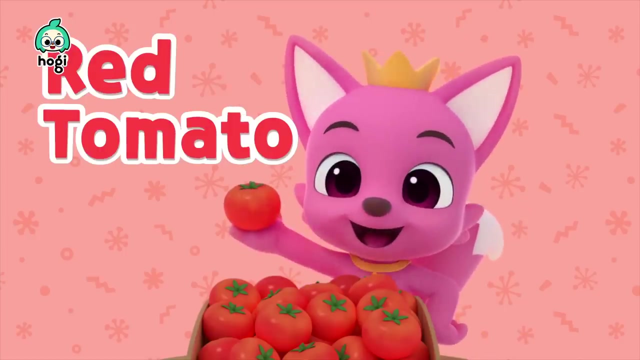 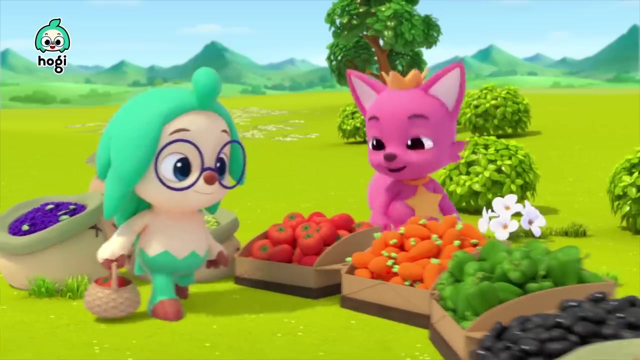 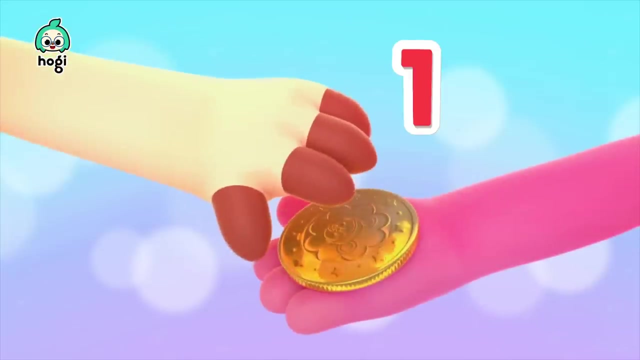 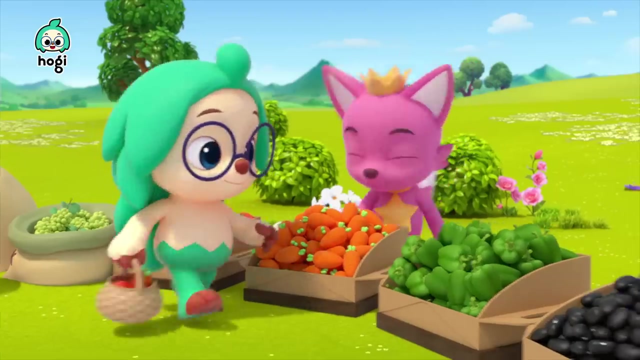 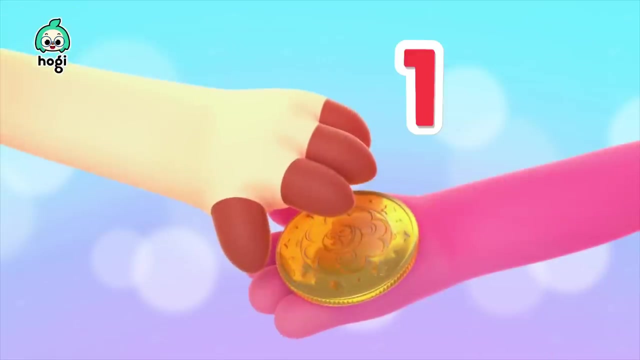 If a woodchuck could chuck wood. If a woodchuck could chuck wood, We did it. Yay. Red, Red tomato One One. Orange, Orange carrot One, Two, One Two. Green Green pepper One. 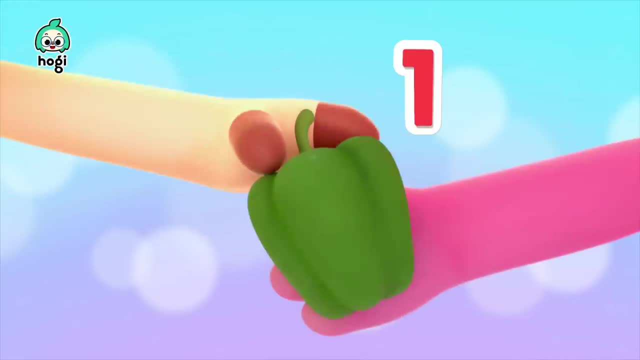 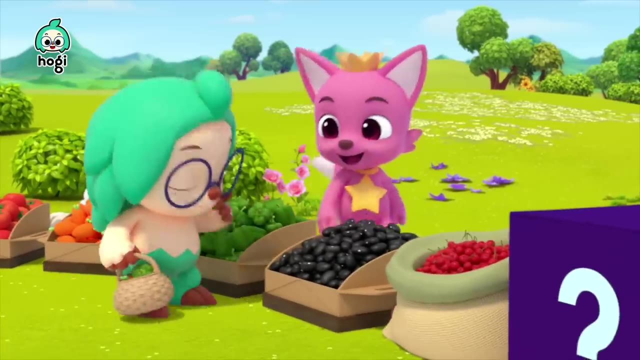 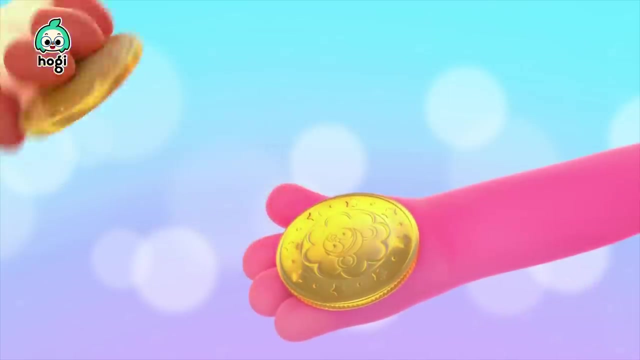 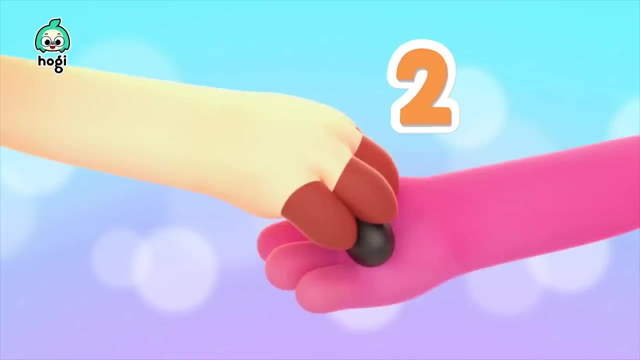 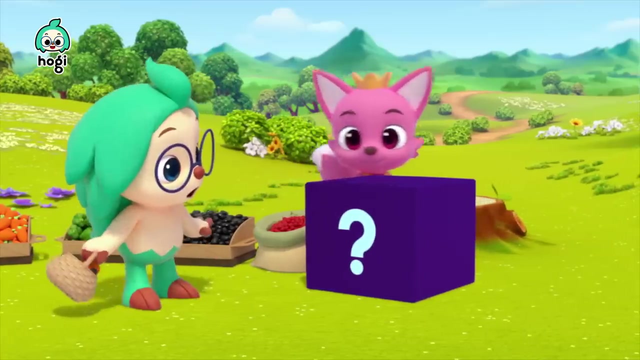 Two, Two, Three. One Two, Two, Three. Black Black bean One One, Two, Two, Three, Three Four. One, One, Two, Two, Three, Three, Four One Two. 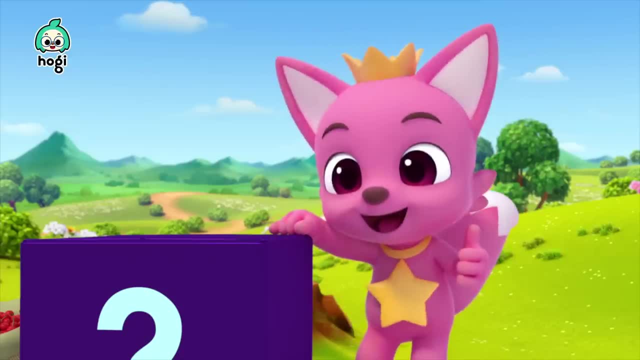 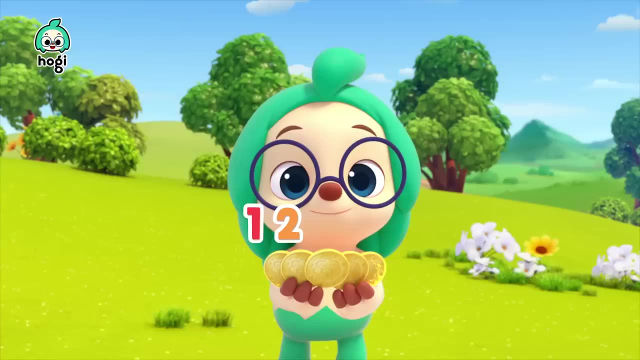 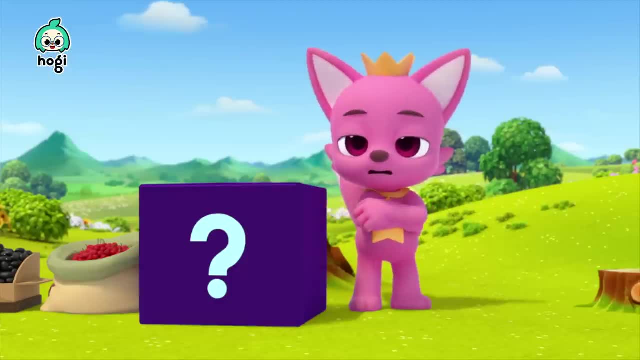 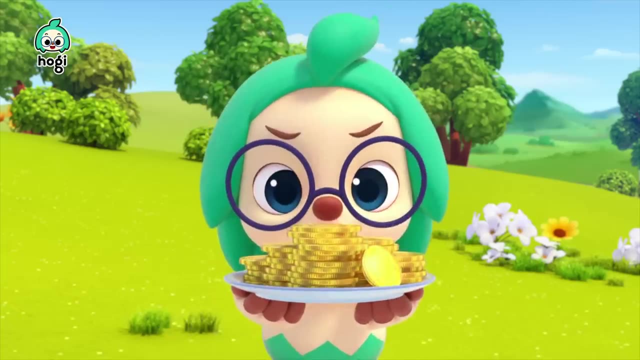 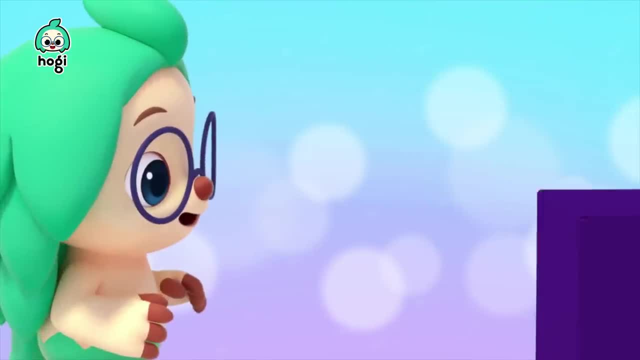 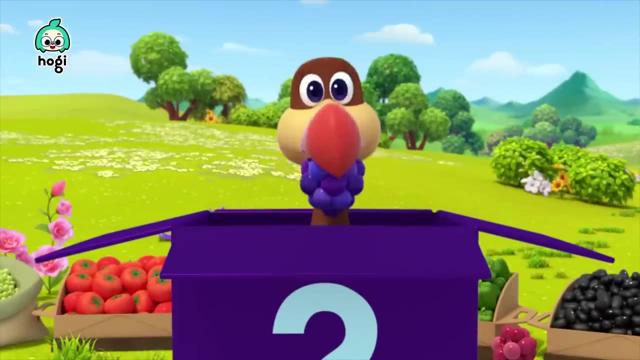 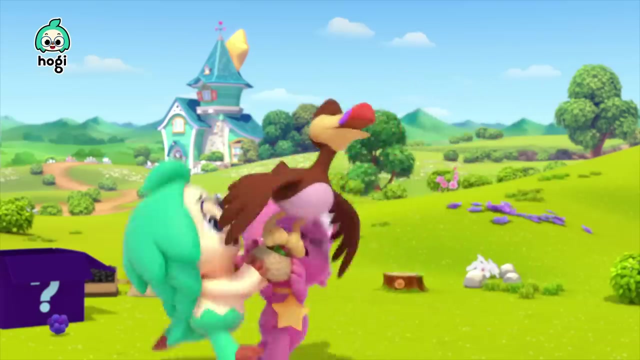 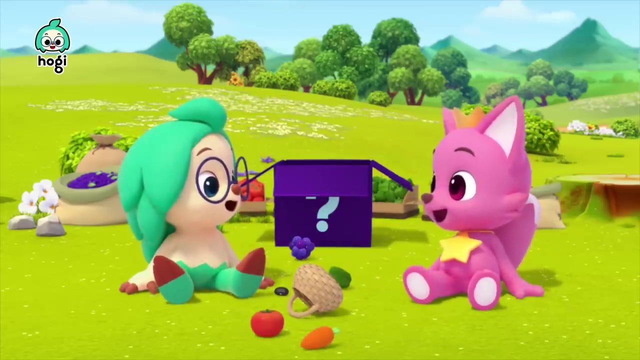 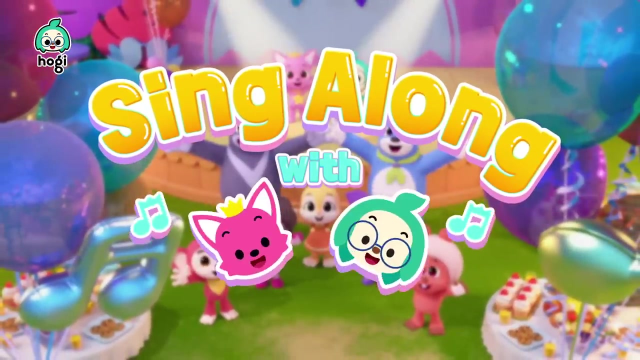 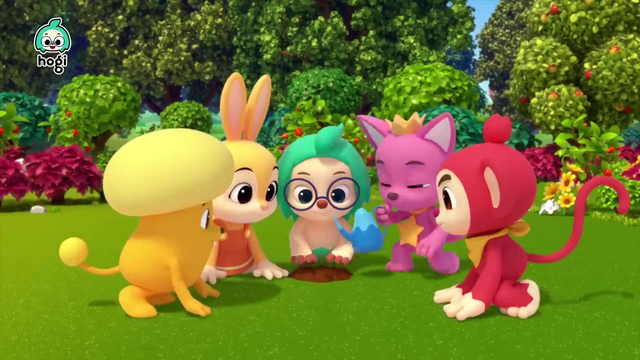 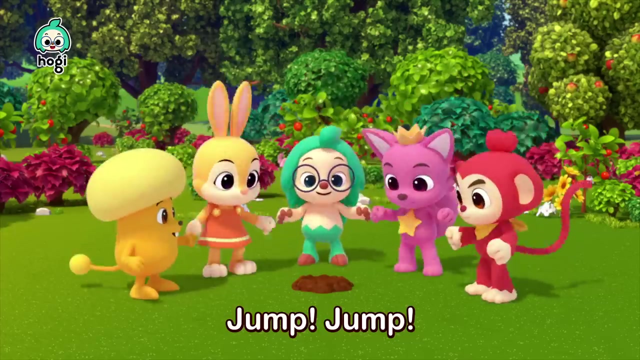 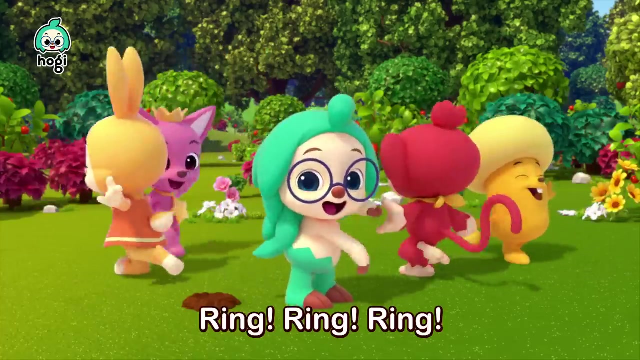 One, Two Sing, along with Ping Pong and Hoagie. Ring-a-ring-a-roses pocket full of posies, Jump, Jump, We all fall down Ring-a-ring-a-ring-a-ring-a-ring-ring-ring, Ring-a-ring-a-ring-a-ring-a-ring-ring-ring. 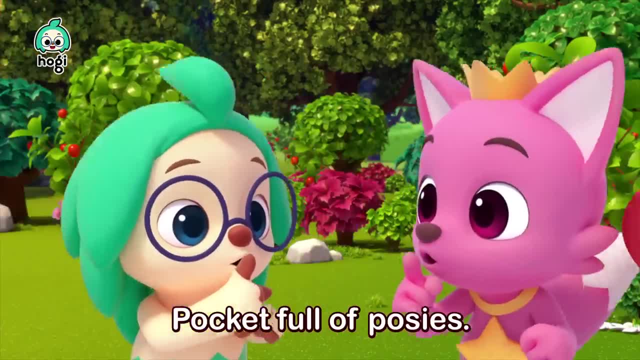 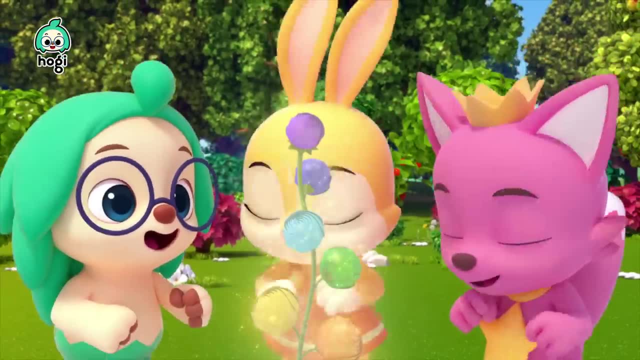 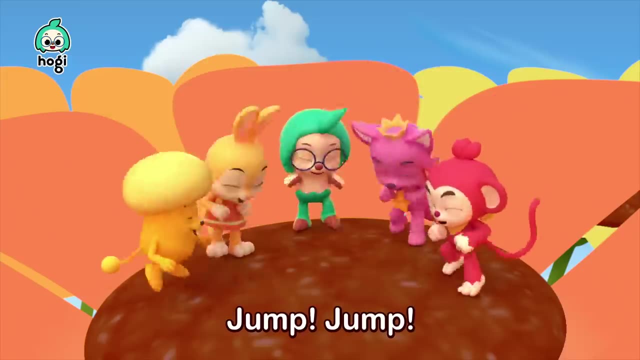 Ring-a-ring-a-roses pocket full of posies- Jump Jump. We all fall down. Ring-a-ring-a-roses pocket full of posies: Jump Jump. We all fall down. Ring-a-ring-a-ring-a-ring-a-ring-ring-ring. 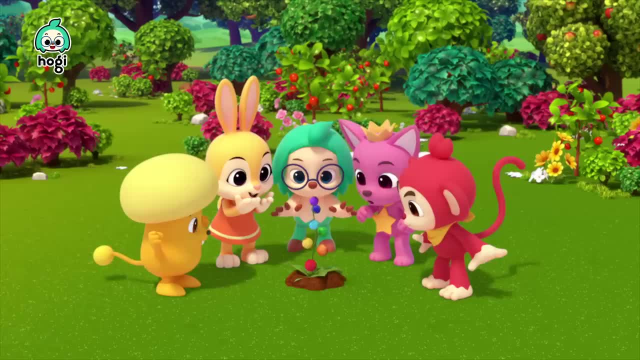 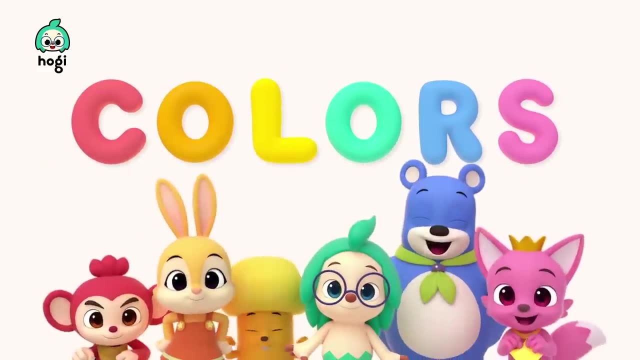 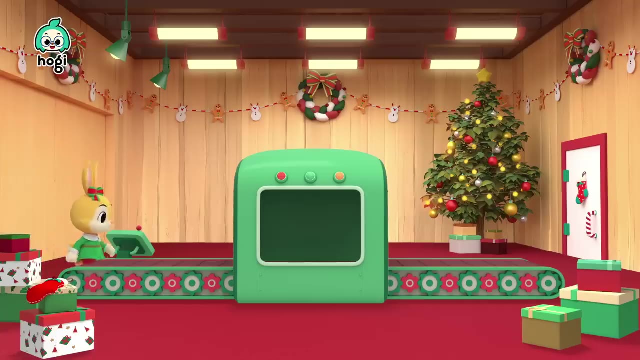 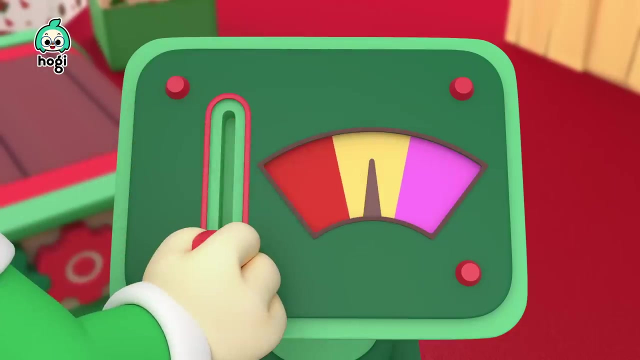 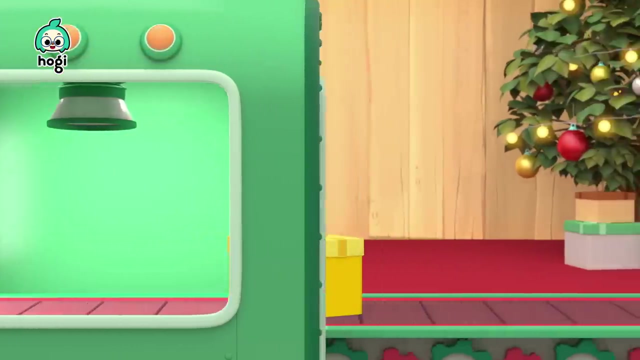 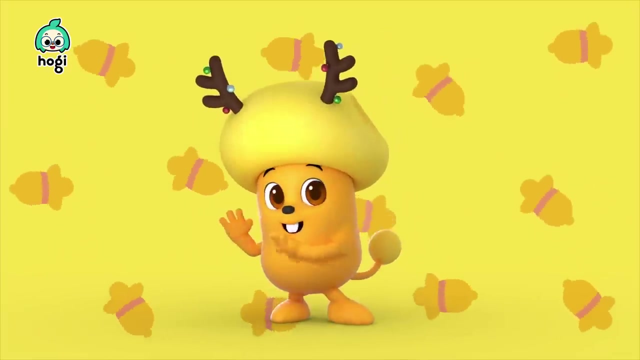 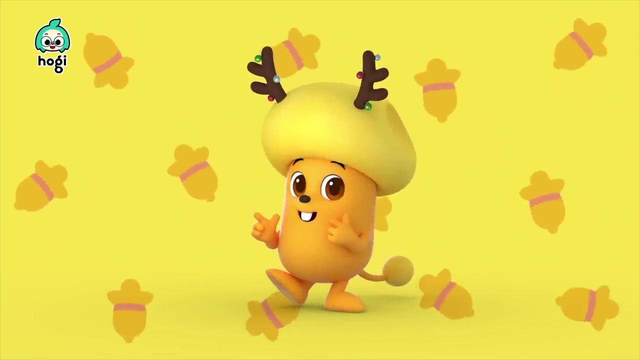 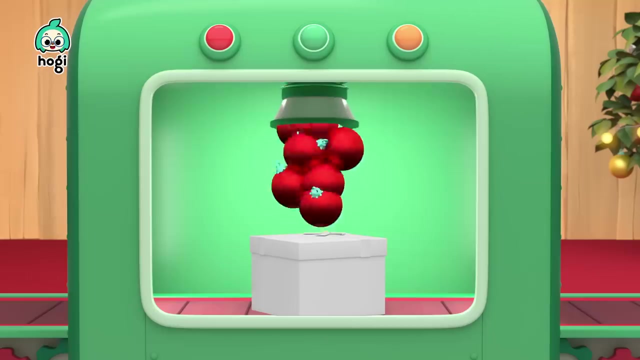 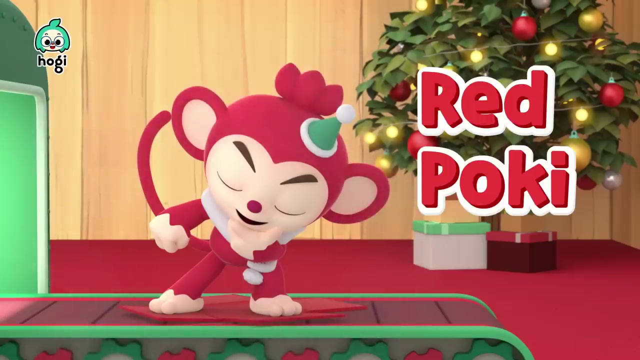 Ring-a-ring-a-ring-a-ring-a-ring-ring-ring. LOL Colors, LOL. Yellow Mayan, Yellow Mayan, Jingle bells, jingle bells, jingle all the way. Oh, what fun it is to ride in a one-horse open sleigh: Red Pokey. 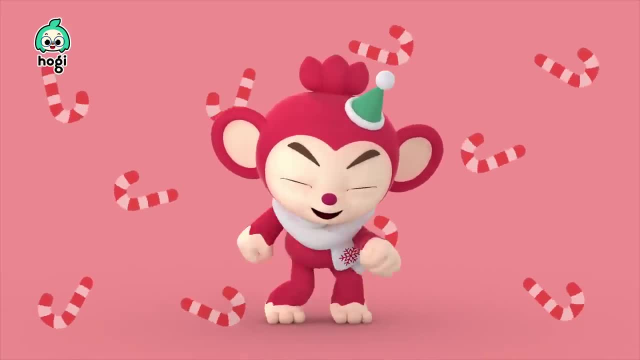 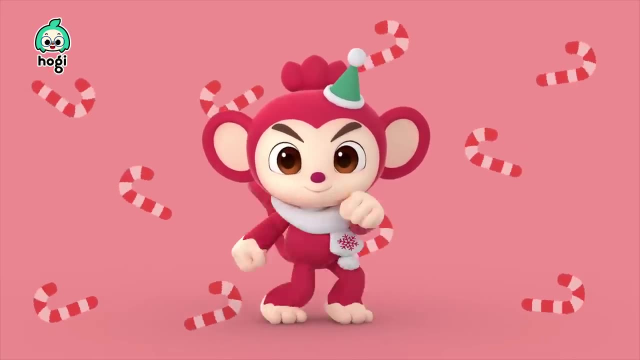 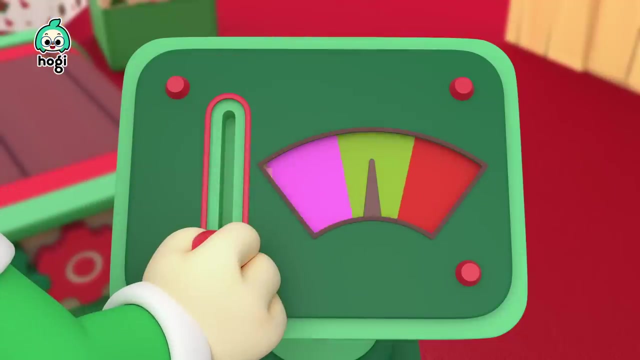 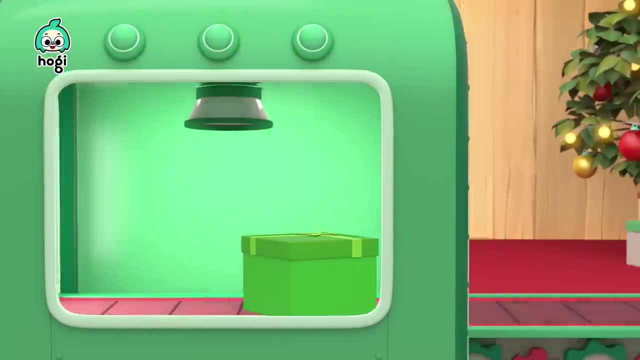 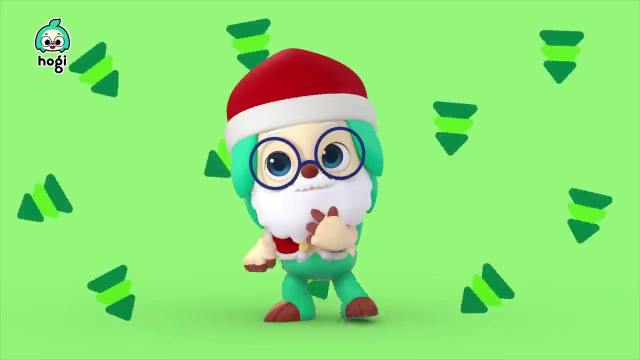 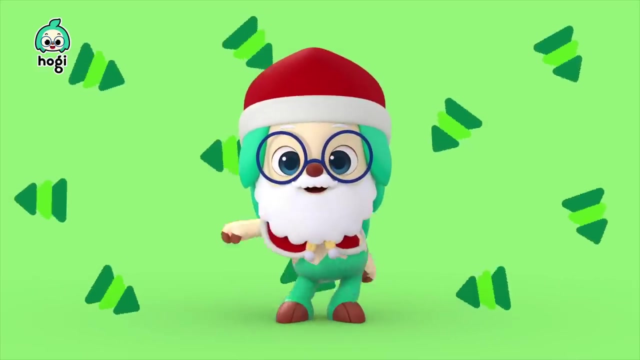 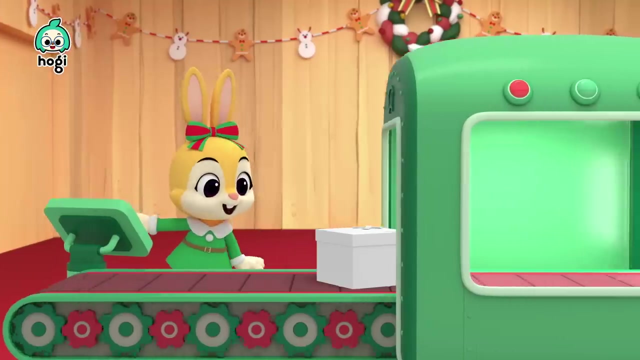 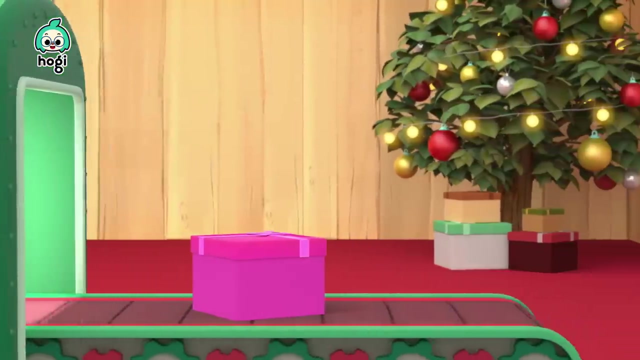 Everybody Twistmas, sing and dance with me. Here we go. Merry, merry, Twistmas. Yeah, Green Hoagie, S-A-N-T-A, S-A-N-T-A, S-A-N-T-A. and Santa is his name-o Pink Pinkfong. 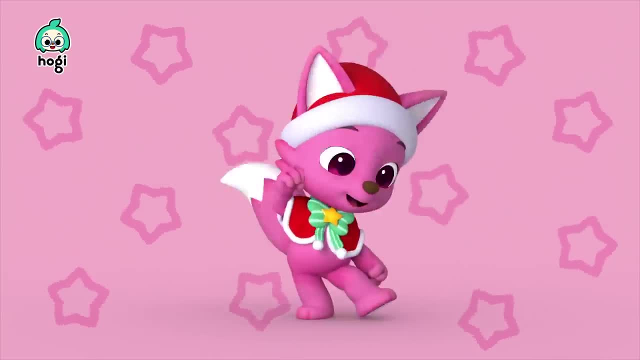 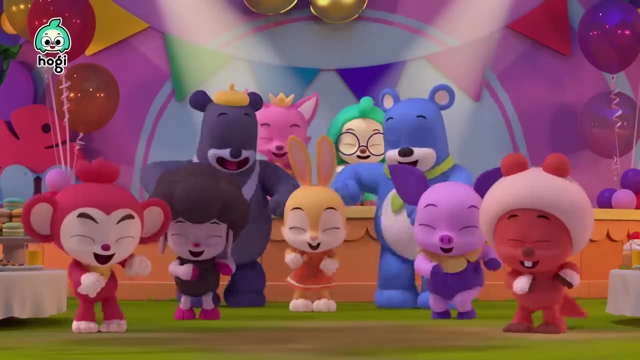 Jolly, jolly doo-doo-doo, jolly, jolly doo-doo-doo, Happy, happy doo-doo-doo, Poi poi, Pinkfong. Sing along with Pinkfong and Hoagie. 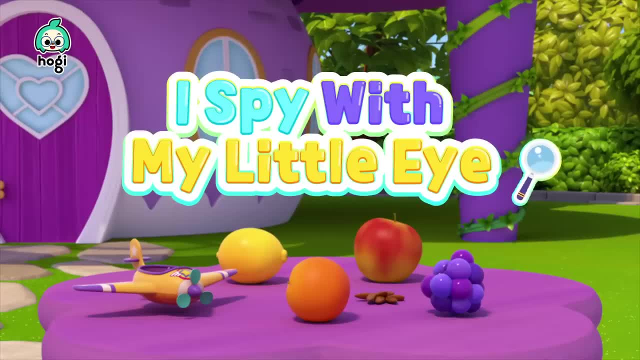 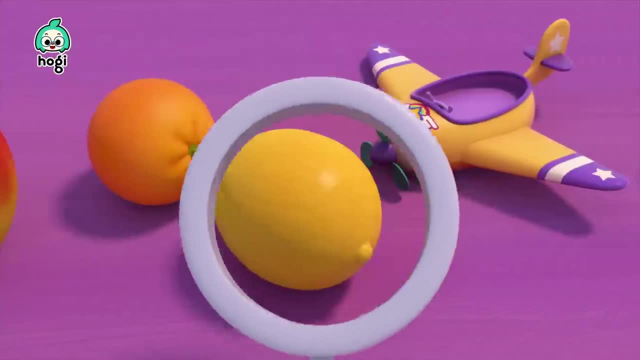 Happy happy doo-doo-doo. do-doo-doo. Happy happy doo-doo-doo. do-doo-doo. Happy happy do-doo-doo do-doo-doo. Happy happy do-doo-doo do-doo-doo. 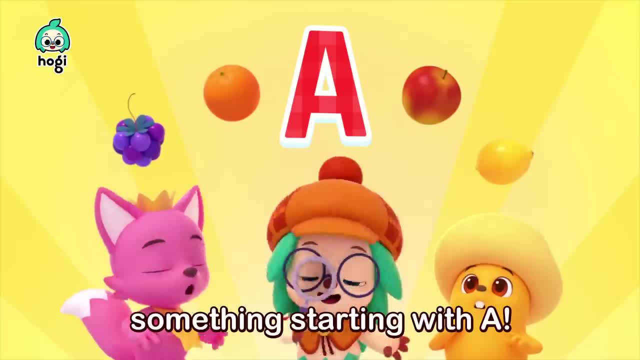 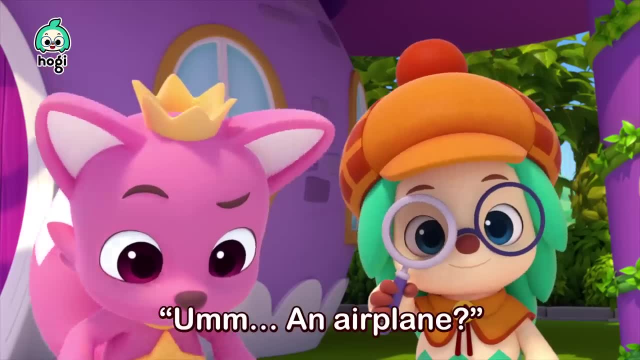 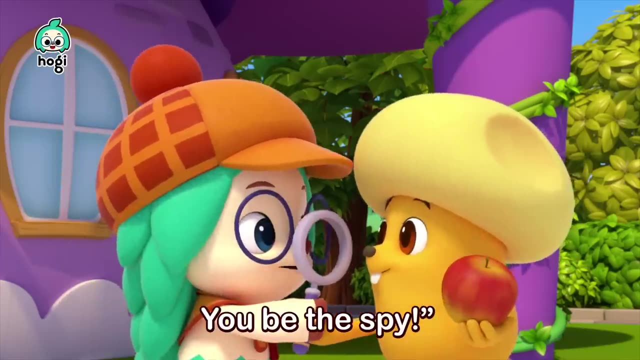 Poi, Poi Poi. I spy with my little eye Something starting with A. I spy with my little eye, Guess what it is. Um, an airplane, Wrong, An apple. You're right, You be the star. I spy with my little eye something starting with E. 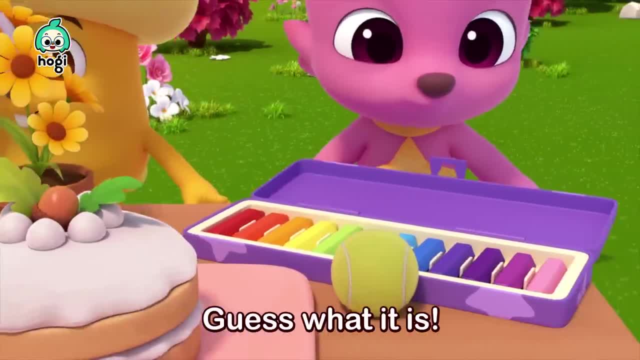 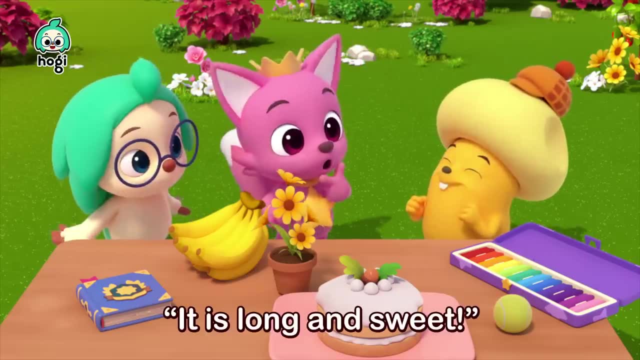 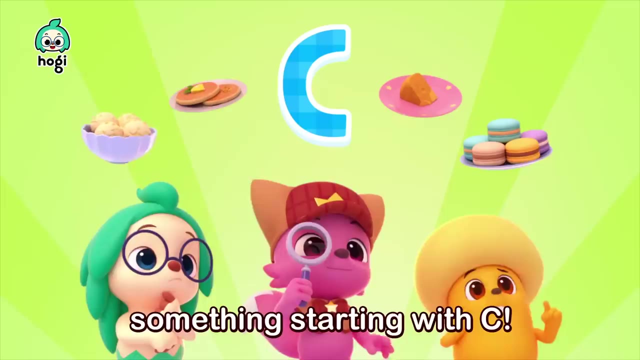 I spy with my little eye. guess what it is. Give us a hint, please. It is long and sweet. Ah, banana, right, Yes, now it's your turn. I spy with my little eye something starting with E. I spy with my little eye. guess what it is. 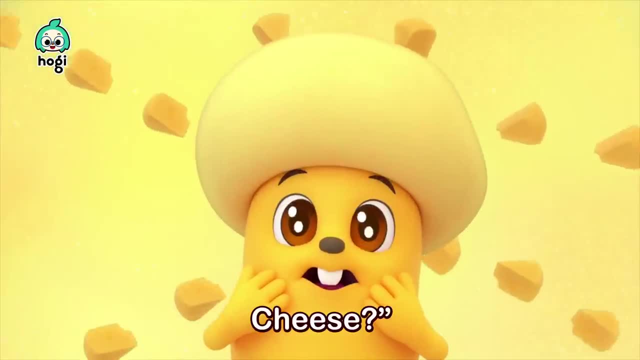 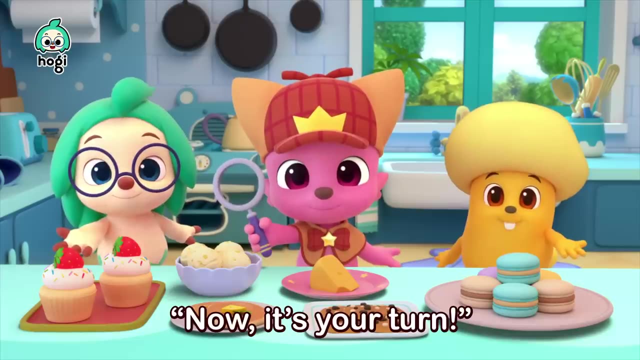 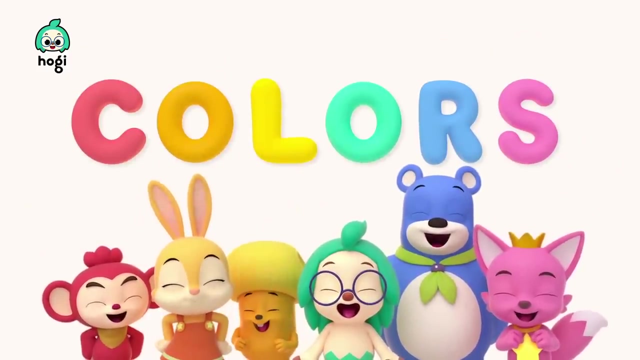 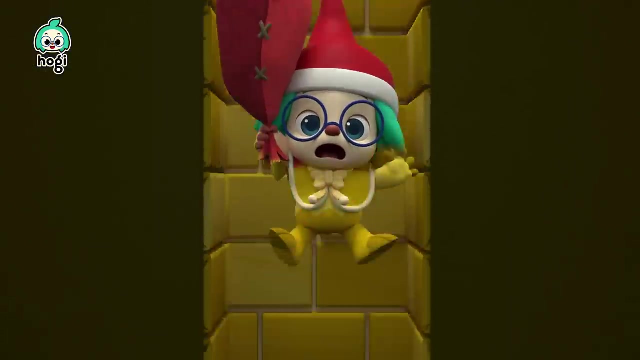 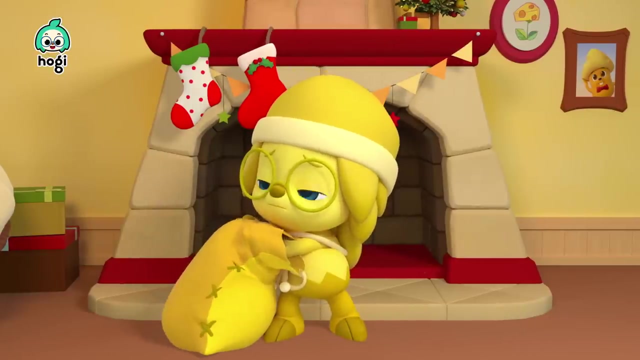 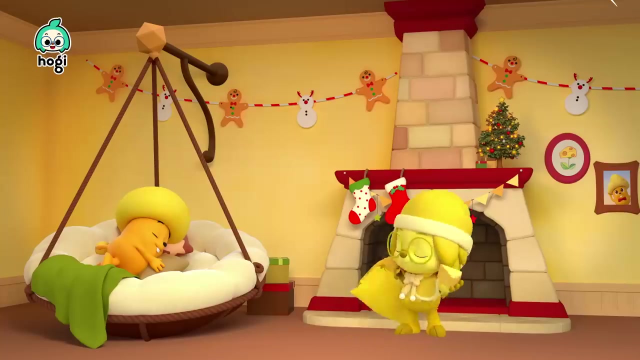 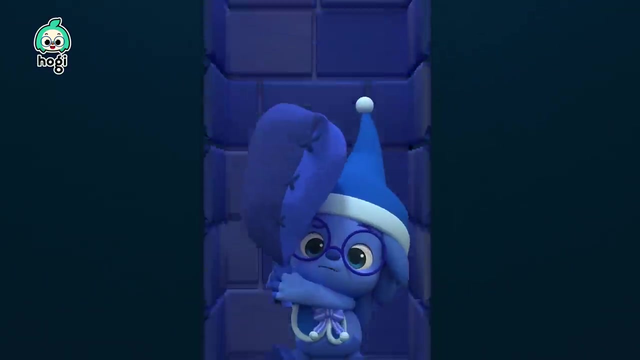 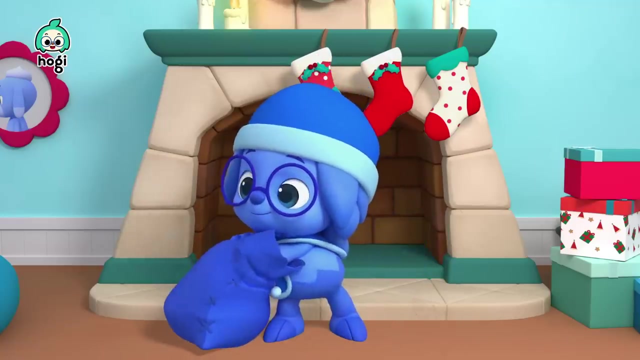 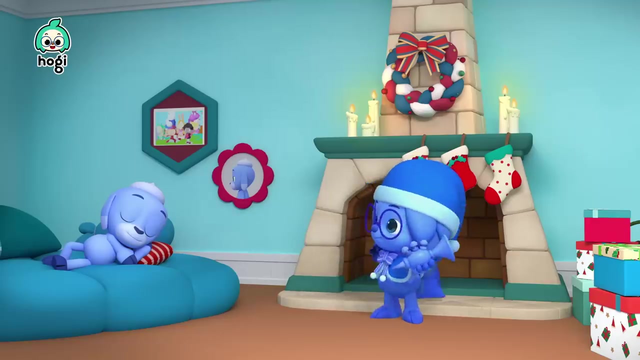 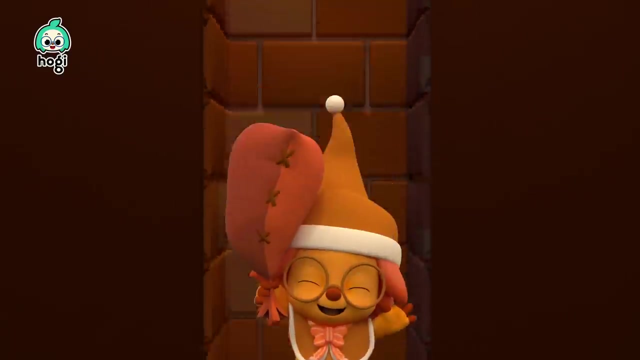 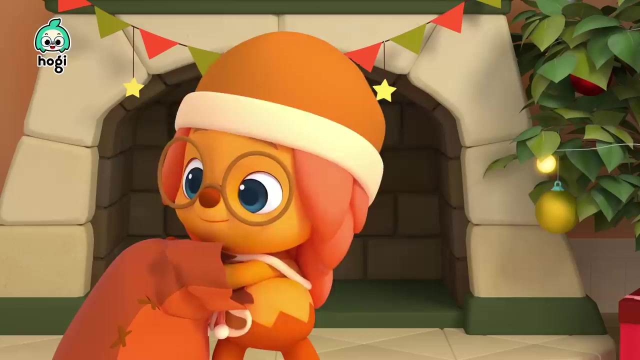 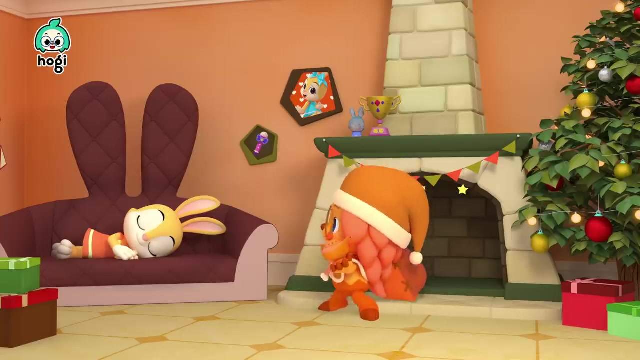 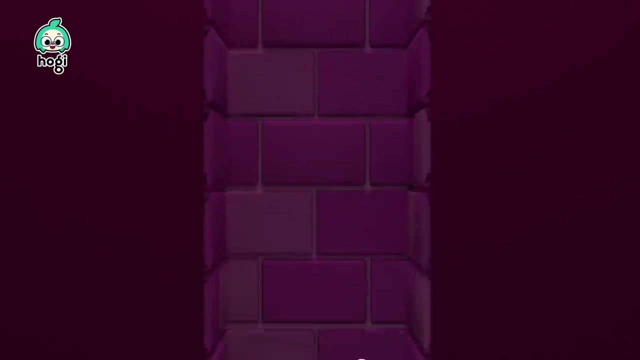 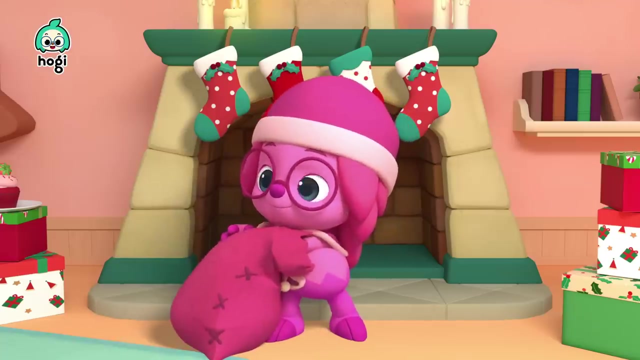 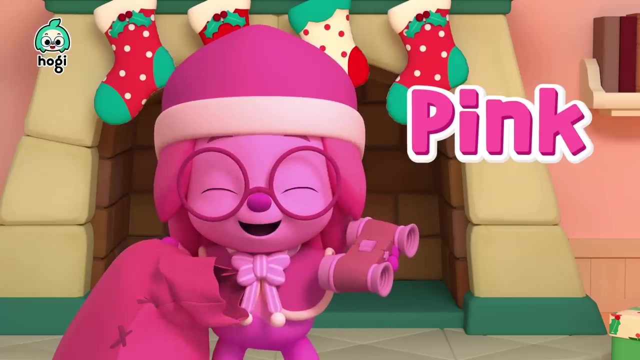 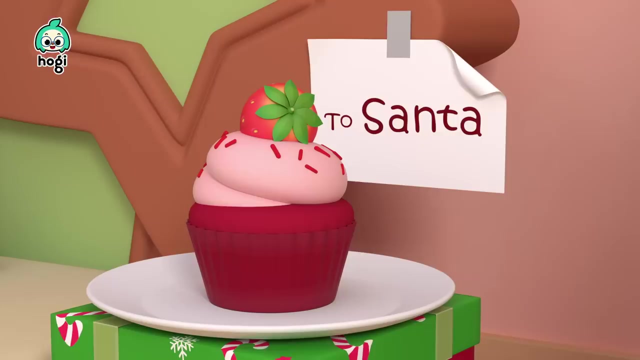 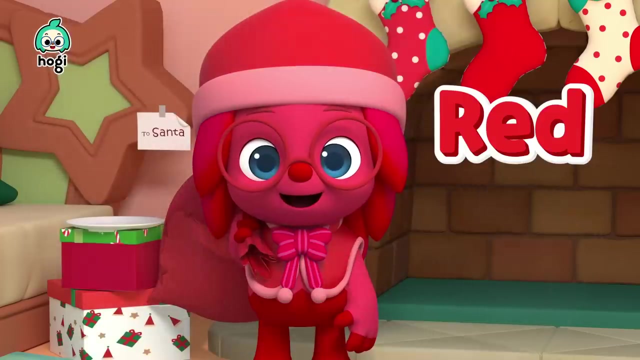 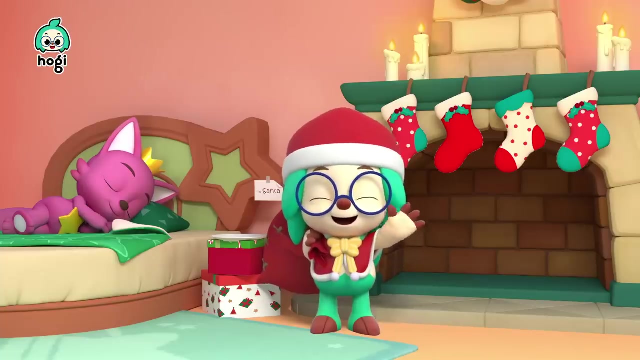 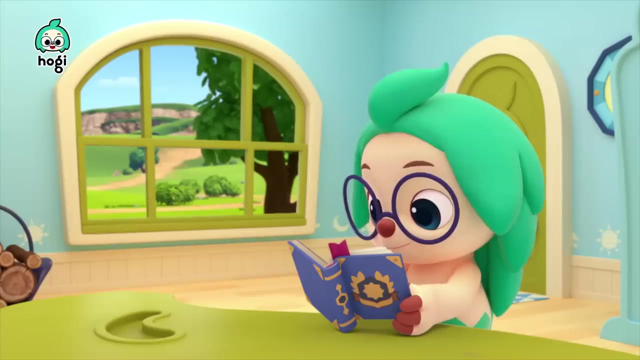 Let me see, is it cheese? Yes, Now it's your turn. Wow, Yellow, Yellow, Yellow, Huh Huh, Oh Hmm. Blue, Orange, Pink, Red Sing along with Pinkfong and Hoagie. Knock, Knock, Knock. 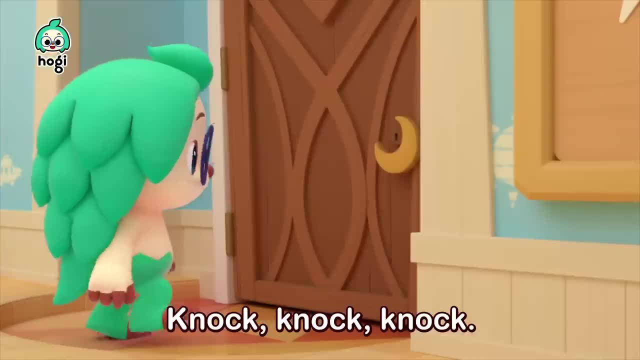 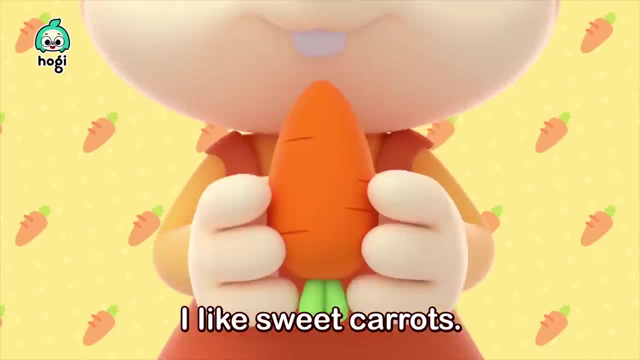 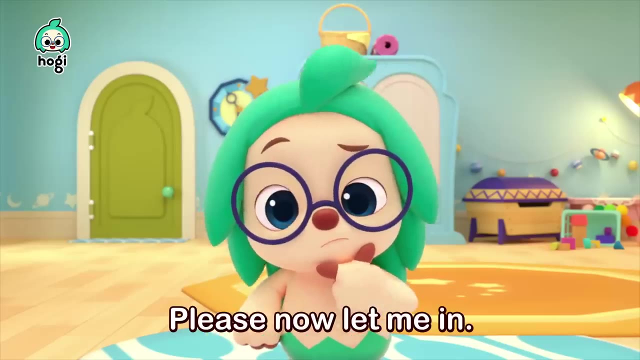 Who's there? Knock, Knock, Knock. Who's there? I have two long ears. I have a short tail. I like sweet carrots. I have big front teeth. I'm good at jumping. Hoagie, I'm your friend. Please now let me in. Aha, Jenny the bunny. 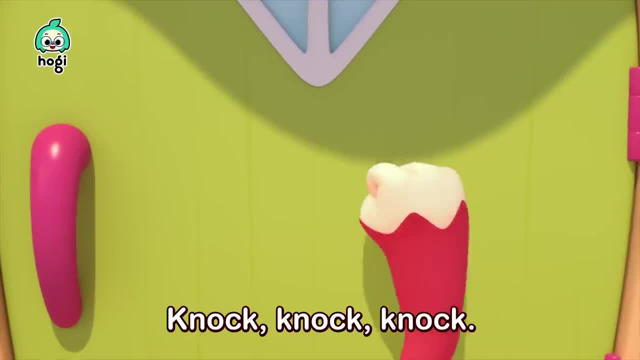 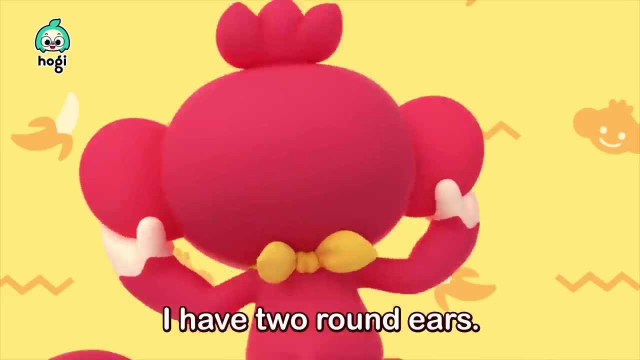 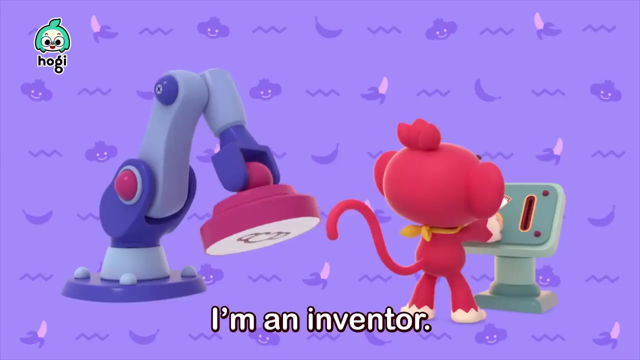 Yes, it's me. Come in. Knock, Knock, Knock, Who's there? Knock, Knock, Knock. Who's there? I have two round ears, I have a long tail, I like bananas, I hang in a tree, I'm an inventor. Hoagie, I'm your friend. 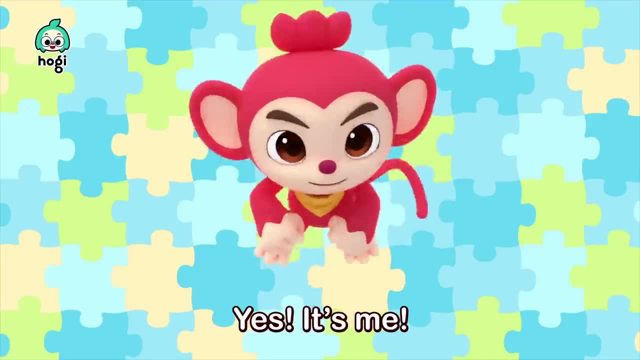 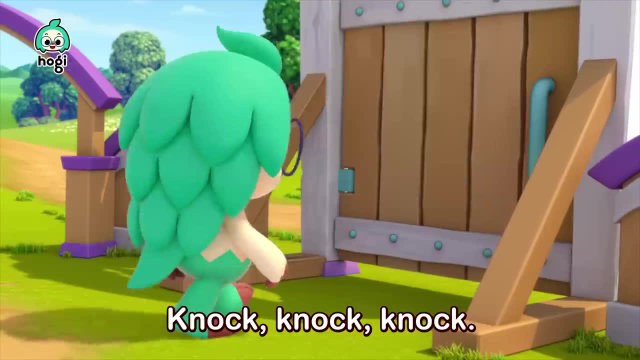 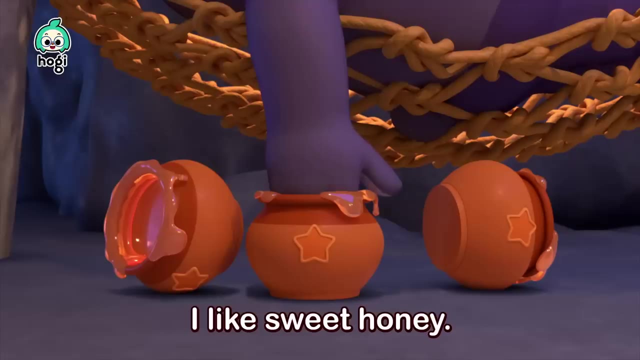 Please now let me in. Hoagie the monkey- Yes, it's me. Come in, Knock, Knock, Knock, Knock, Knock, Who's there? Knock, Knock, Knock, Who's there? I have two small ears. I have big grey paws. I like sweet honey. 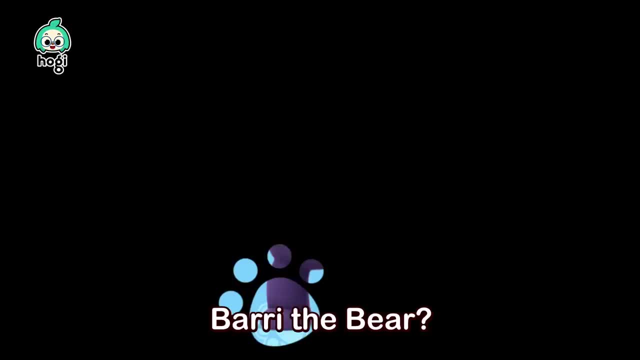 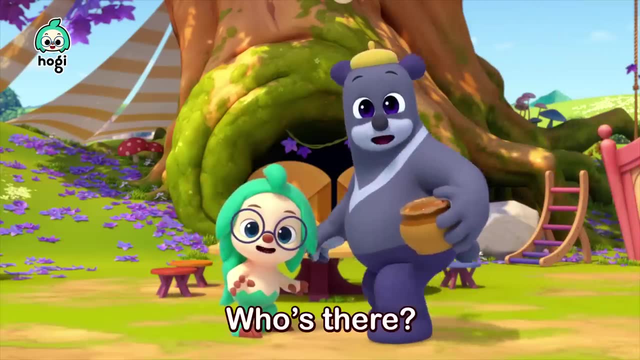 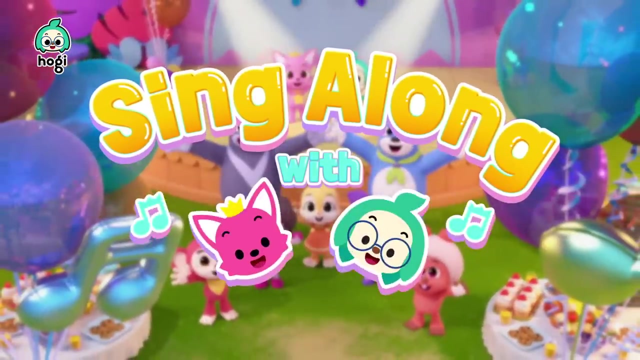 I sleep in winter. I'm mighty and strong. Hoagie, I'm your friend. Please now let me in. Hoagie the bear- Yes, it's me. Come in, Knock, Knock, Knock. Sing along with Ping Pong and Hoagie. 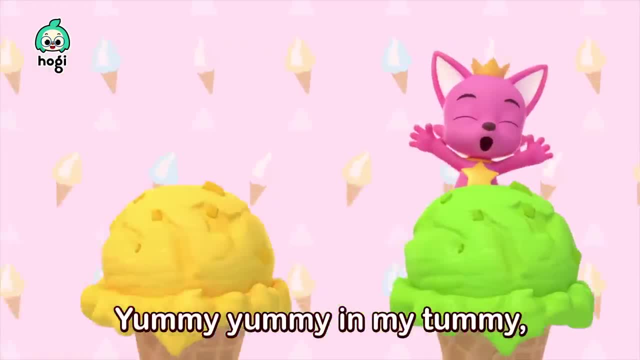 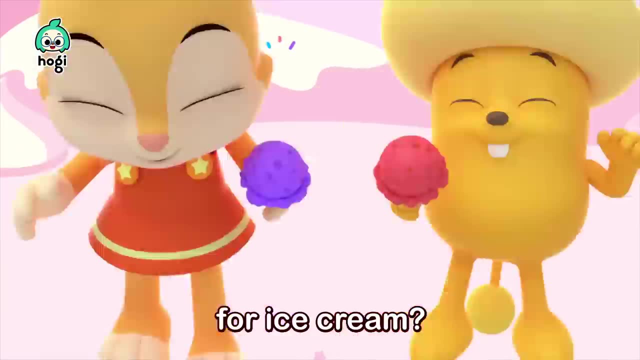 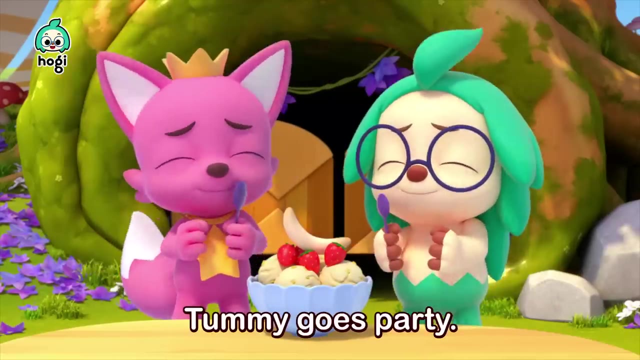 Ice Ice Ice Icecream. Yummy, Yummy in my tummy. Ice cream. ha Ice Ice, Ice Icecream. Are you ready to scream for Ice cream? Yaaaay, Yum, Yum, Yummy, Tasty Sweet Woo Tam Tam. Tommy Goes Party. 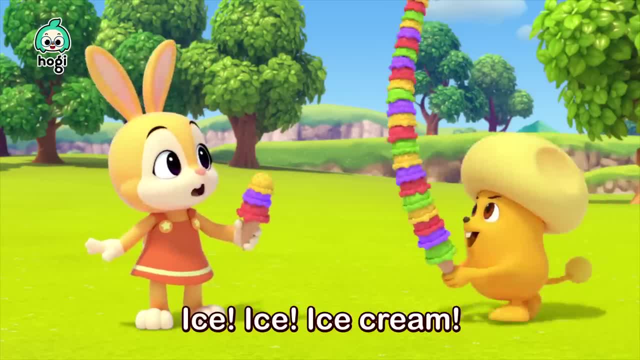 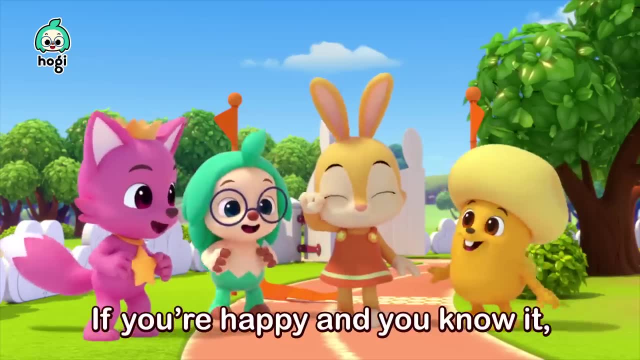 Woo Ha, This is my favorite treat. Ooh yeah, Ice, ice, ice cream When the day is hot and steamy. Ice cream If you're happy and you know it. Ice cream, Don't let it melt away. wake it up. 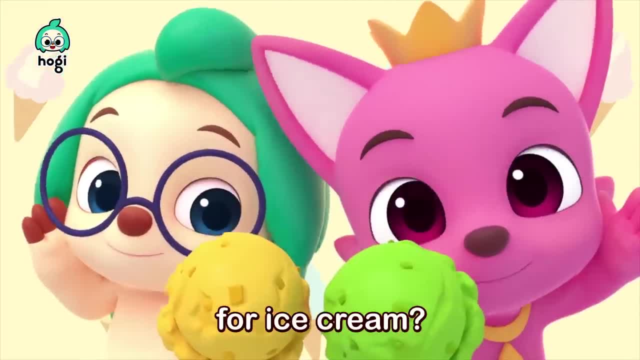 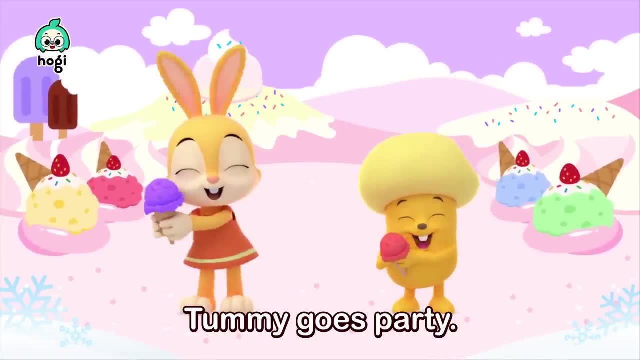 Ice cream. Are you ready to scream for ice cream? Yay, Yum yum, yummy, tasty, sweet Tongue. tongue. tummy goes party. This is my favorite treat. Ooh yeah, Ice, ice, ice cream. 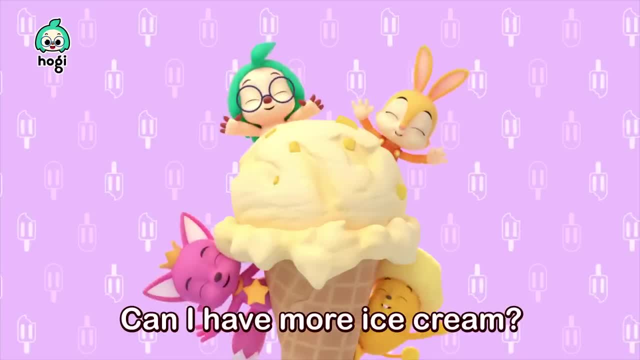 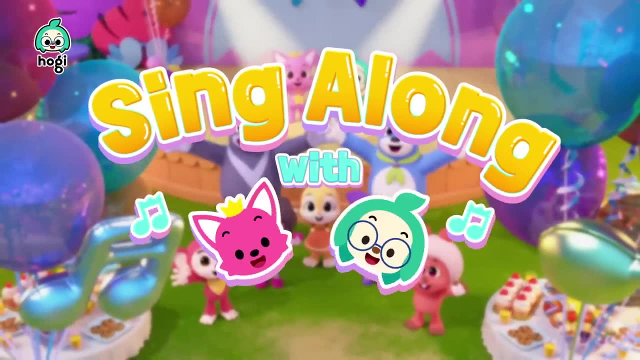 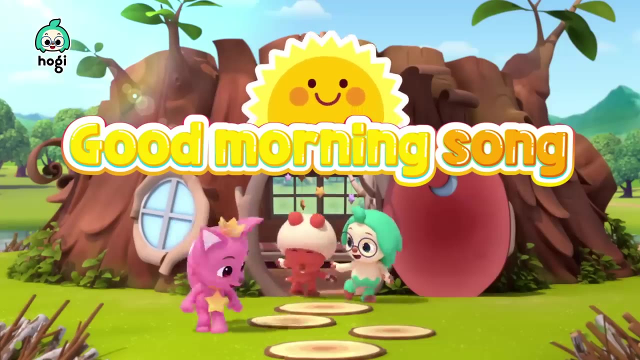 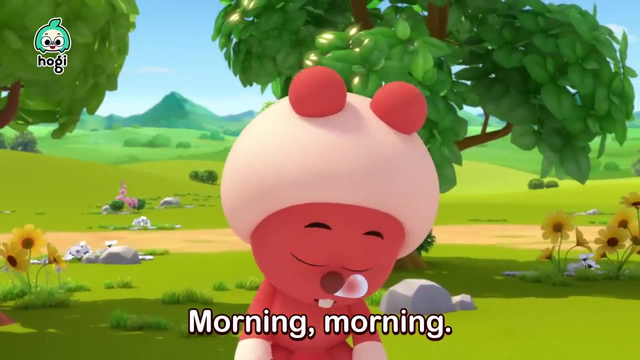 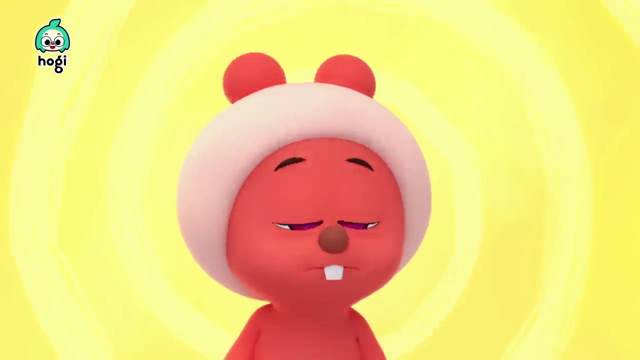 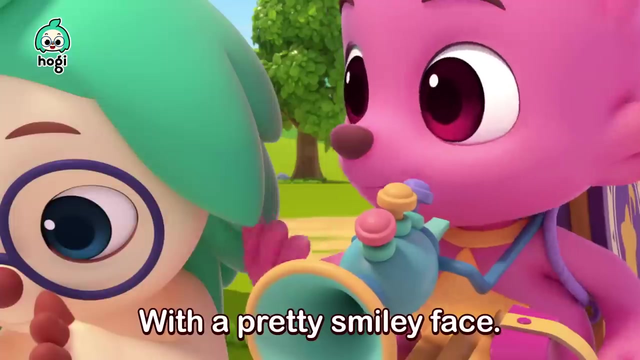 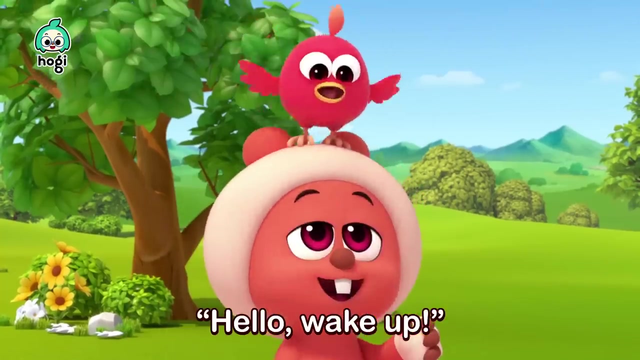 Can I have more ice cream When the sunny sun comes up? Morning morning, it's morning, With a pretty smiley face. Morning morning, it's morning. Hey, The birds chirp, chirp, Hello, wake up. 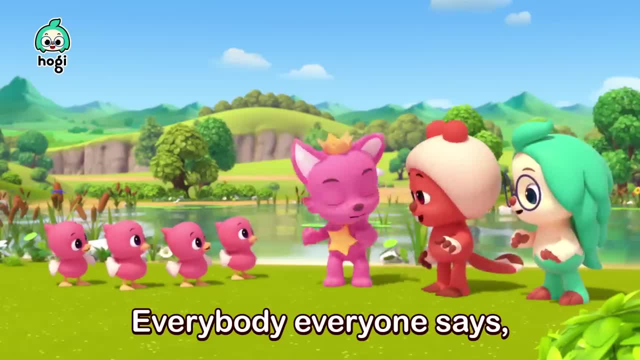 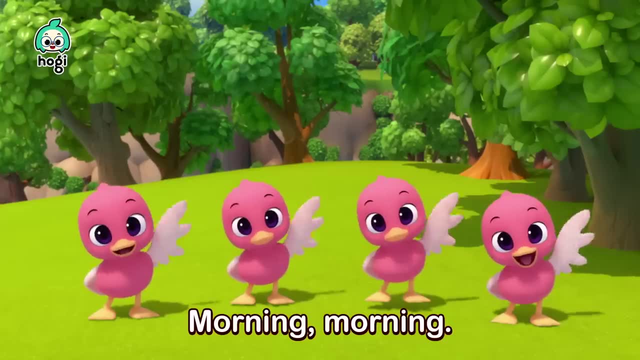 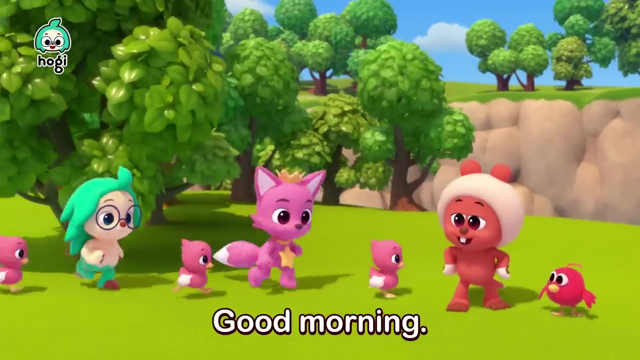 The ducks quack, quack, Hello, get up Everybody. everyone says hello. Morning morning, it's morning. Morning morning, good morning, Morning morning. happy morning, Morning morning, shiny morning, Good morning. it's time to wake up. 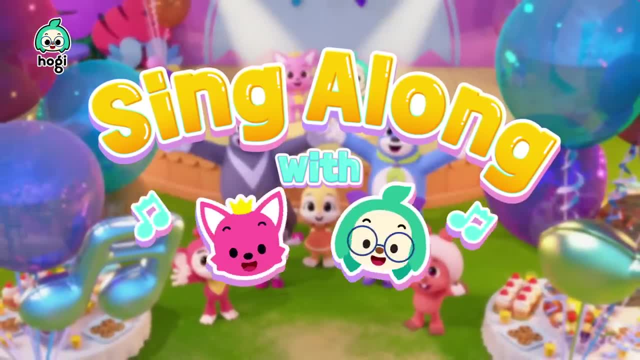 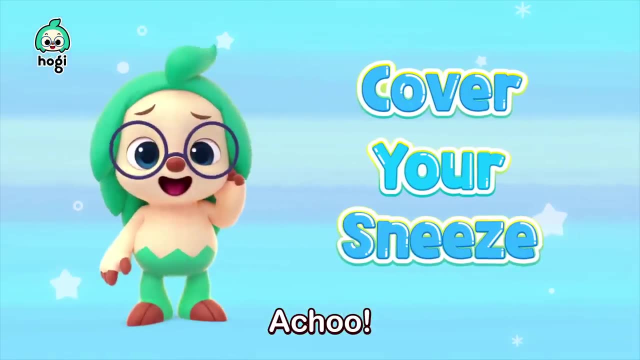 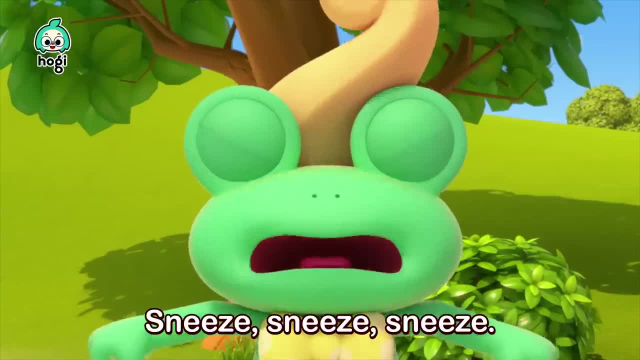 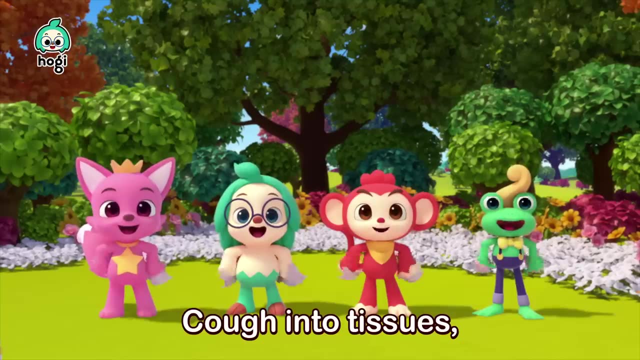 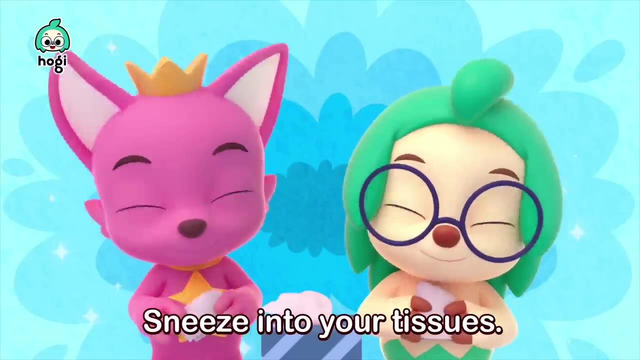 Do not spread your germs. Sneeze, sneeze. When you sneeze, how do you cover your mouth? Grab some tissues, Cough into tissues, Cough into tissues. Sneeze into tissues, Sneeze into your tissues. 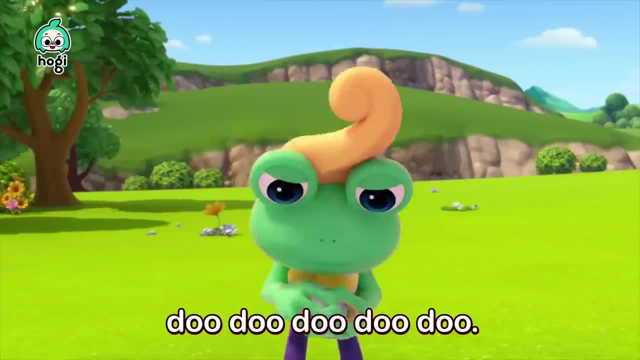 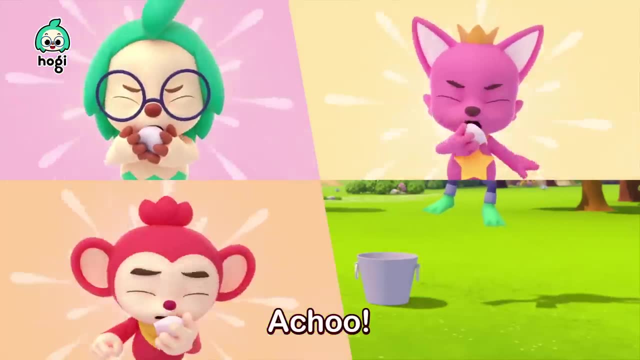 Throw away, Throw away To the trash, To the trash, Yay, Achoo, achoo, achoo, achoo, Cough, cough, cough. When you cough, cover your mouth, Cover your mouth. 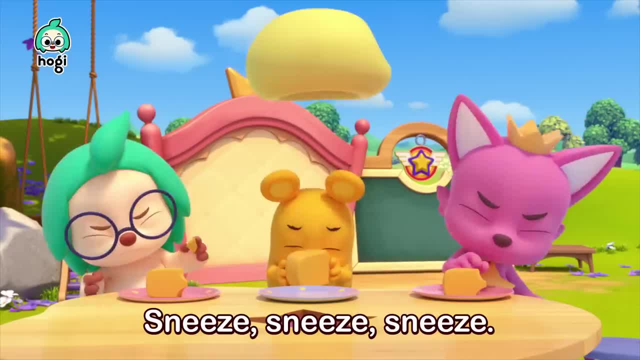 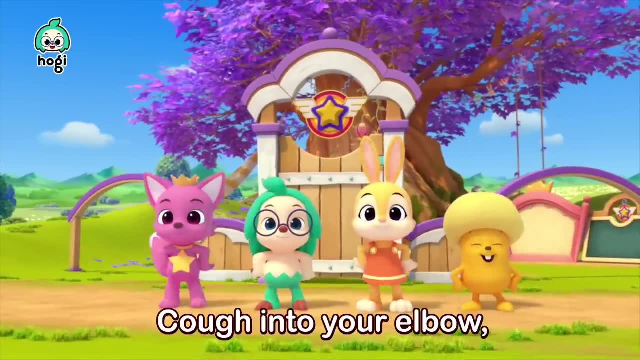 Do not spread your germs. Sneeze, sneeze When you sneeze. what if there are no tissues, Elbows, not your hands. Cough into your elbow, Cough into your elbow, Freund into your elbow. 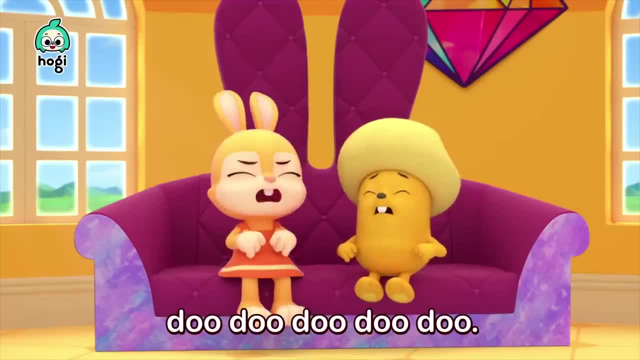 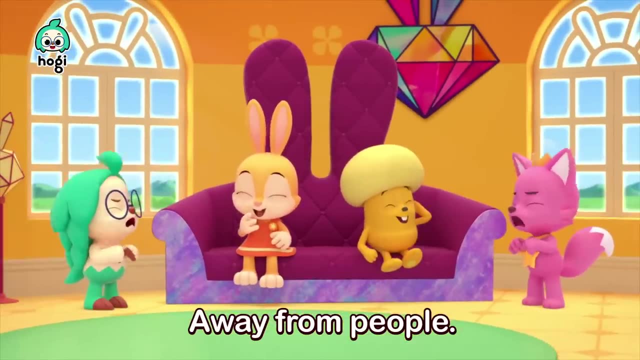 Jealousy to your elbow. Turn your face. Turn your face Away from people. Away from people Only when you're on the phone, Achoo.